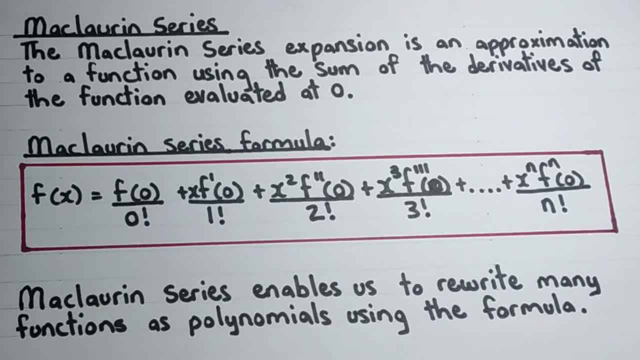 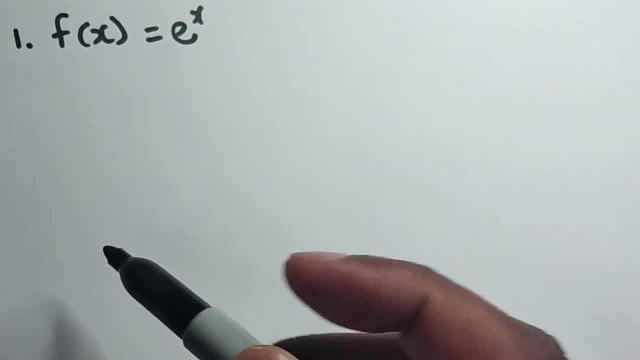 All right, As polynomials. So I'll demonstrate that. Now let's look at how to write MacLaren series. expansion for the function f of x is equal to e to the power of x. All right, So how do we do that? 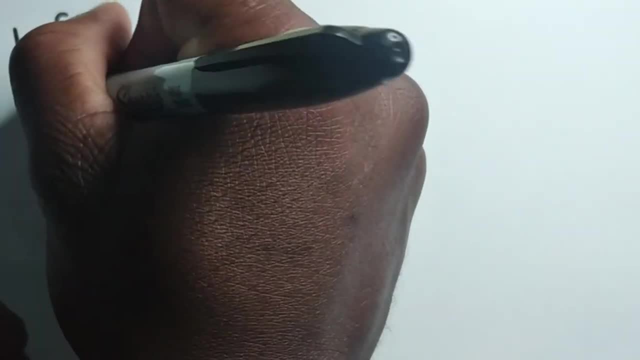 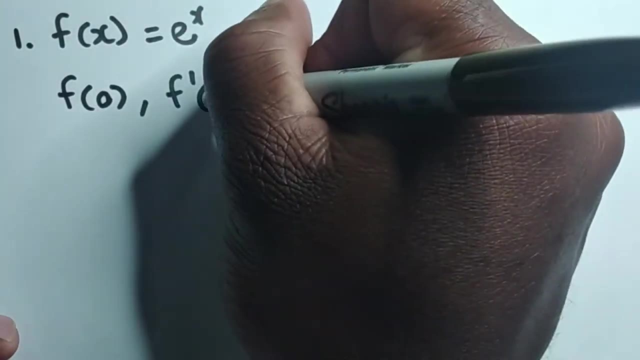 So how do we go about this thing? Now, some of the things that we want to find. we want to find f of zero. We also want to find obtain the result that we'll get after we substitute zero in the first differential of f of x. 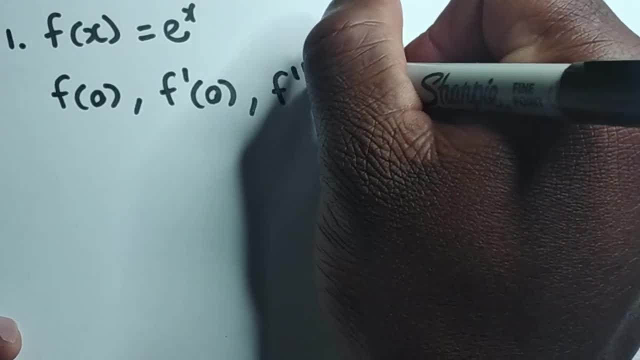 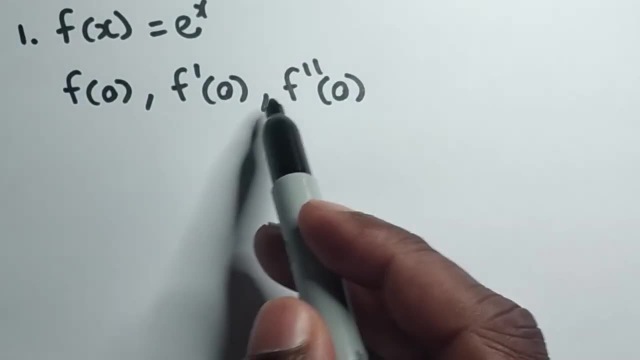 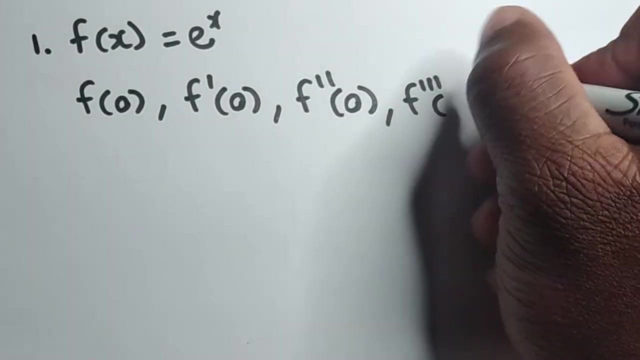 And we'll also want to find the result that we'll get when we substitute zero into the second differential of f of x. All right, If we're going to do three iterations now, if we're going to do more iterations, then you want to find the result that you'll obtain after you substitute zero into the third differential of f of x, and so on and so forth. 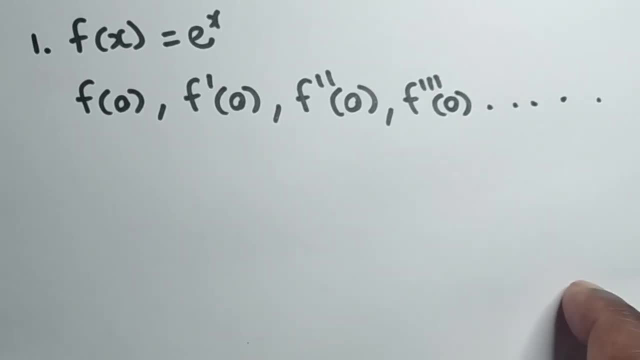 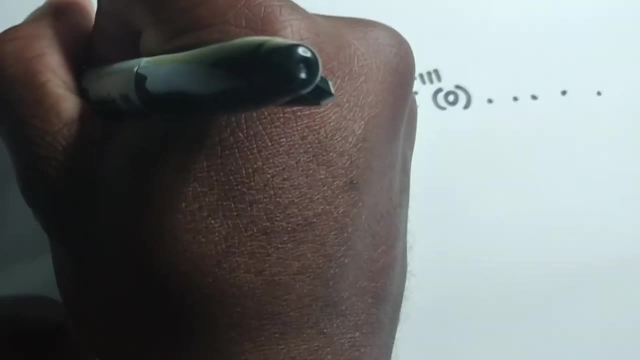 So you can continue this thing. Many more iterations? All right, But we are going to stop at three iterations, So we are going to just look at this part right here so we can complete this video in a timely manner. All right, So what is f of zero? 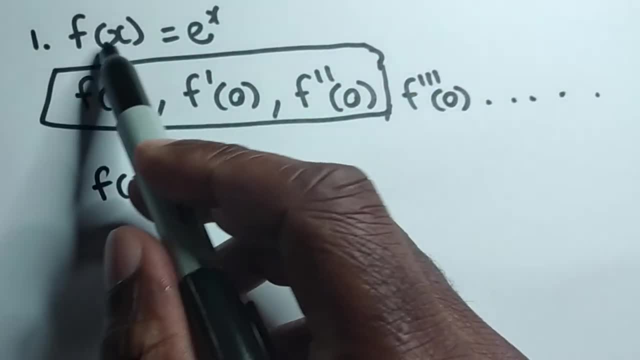 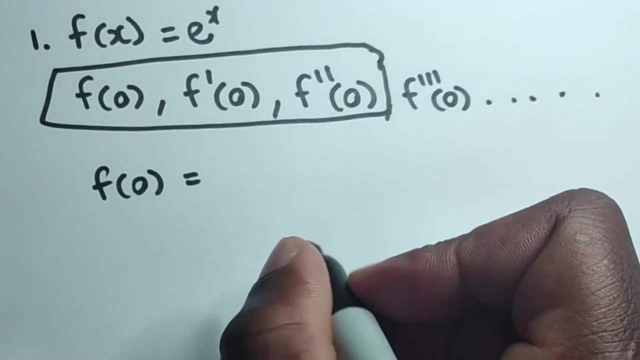 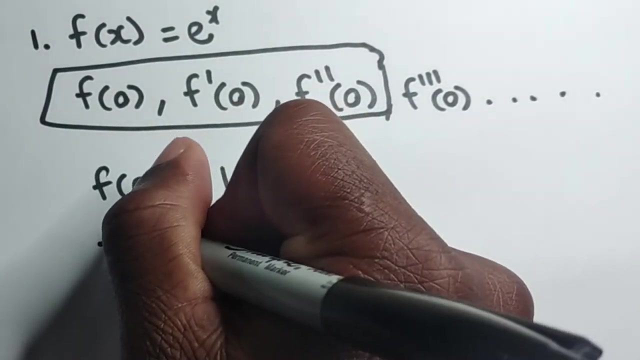 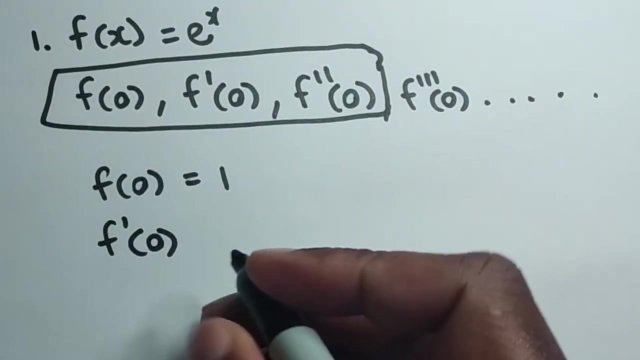 F of zero. What would you get if you subbed? If you replace X with zero, All right, We'll obtain e to the power of zero. Anything raised to the power of zero is one, All right. Now the second thing that we want to find is what. what do you get if you substitute zero into the first differential of f of x? 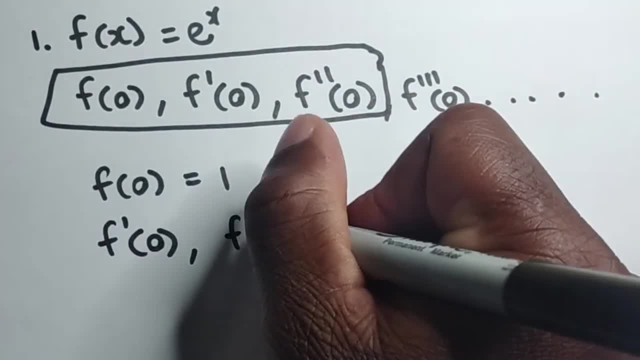 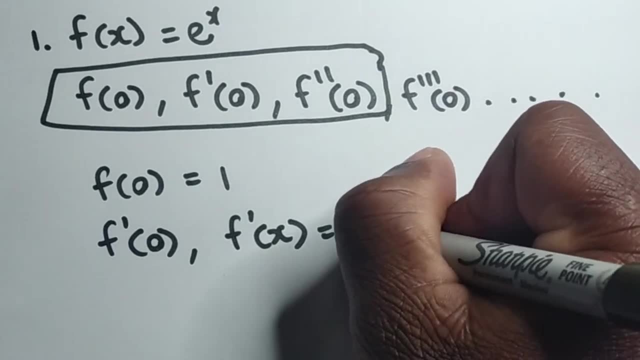 All right. So we need to find the first differential of f of x first. All right, If you differentiate e to the x, you will obtain the The Same result, which is e to the x. All right Now, if you sub. 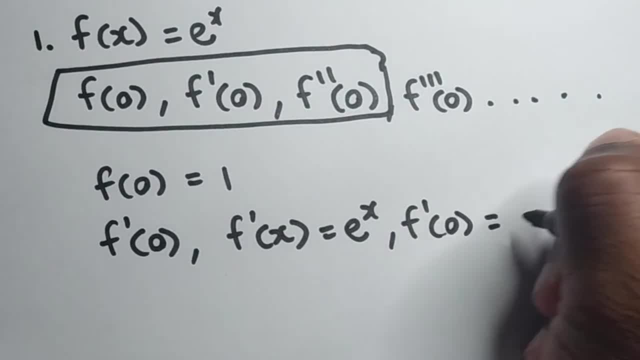 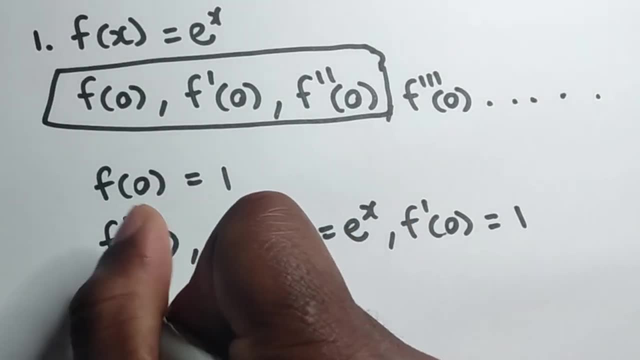 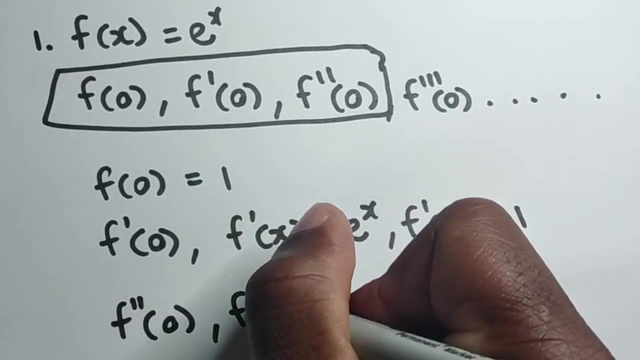 Zero into this function. what will you get? Again? you'll obtain one, All right. So e to the power of zero is one. Now I want to do the final iteration for the sake of this video. So I want to find the second differential of f of x. 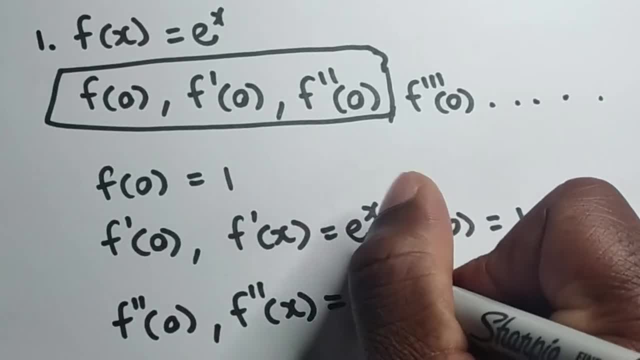 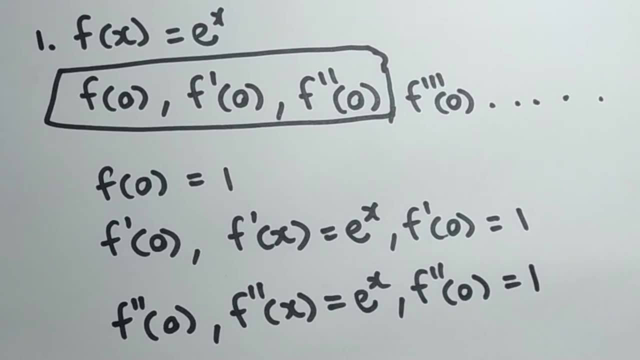 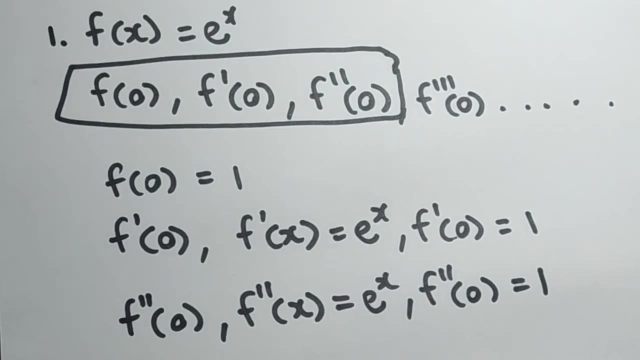 All right. And again, if we differentiate e to the x, we'll obtain the same e to the x. if we sub zero in this thing, again we'll obtain one All right. So what I want to do now is to see how we can plug in these result into the Maclaurin series formula. 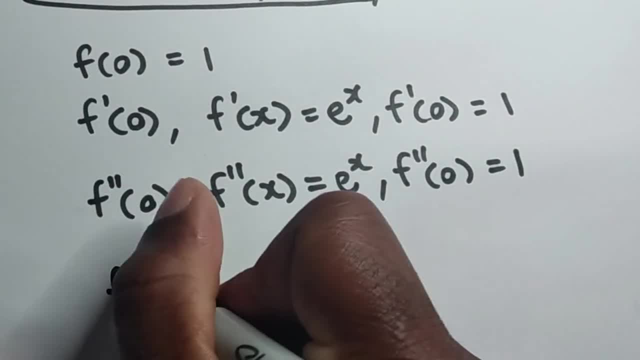 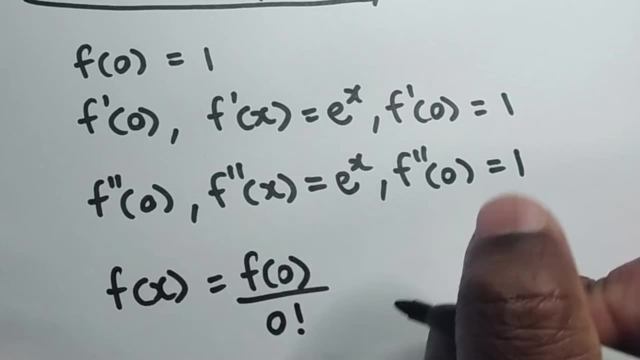 All right, So recall the Maclaurin series. formula f of x is equal to f of zero over zero factorial, plus x times the result that we get when we plug in zero into the first differential of f of x over one factorial, plus x squared times the result that we'll get when we plug in zero into the second differential of f of x over two factorial. 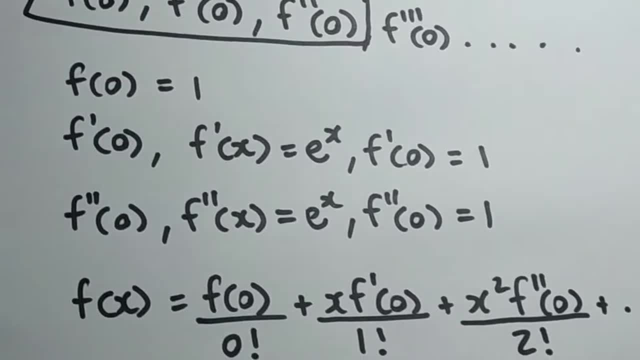 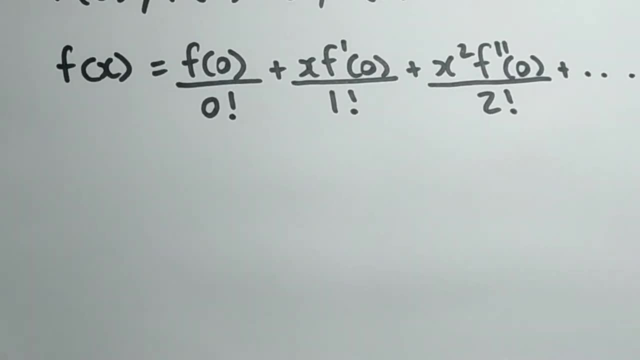 All right. And again, we can't continue this thing, This thing go on and on. All right, So we'll stop right there for the sake of this video Now. So we're going to plug in these values now. So f of x is equal to now. 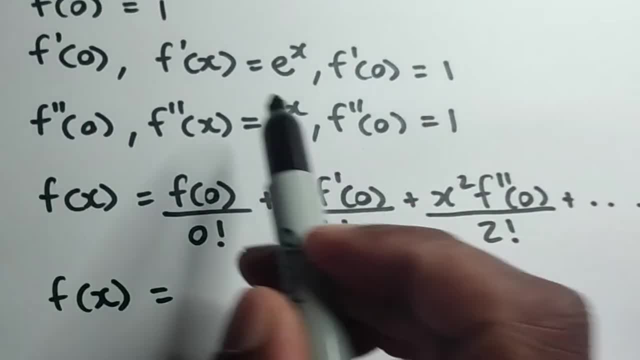 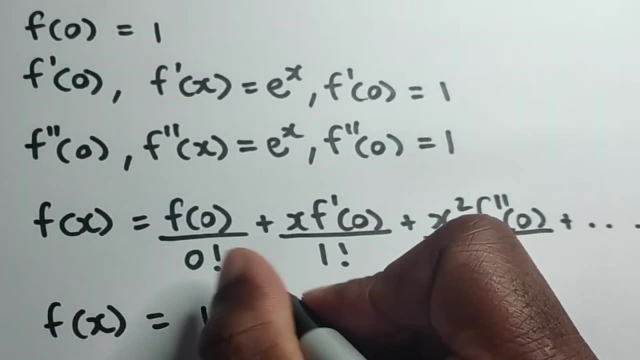 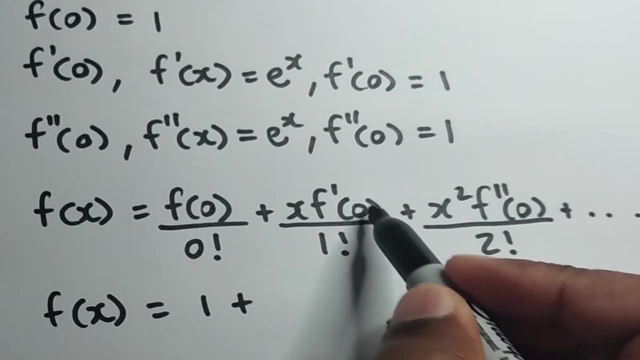 What did we get for for f of zero? The result that we got was one over zero factorial, which is one. So one over one is one. All right, Then we have what x times the result that we got when we substitute zero in the first differential of f of x. 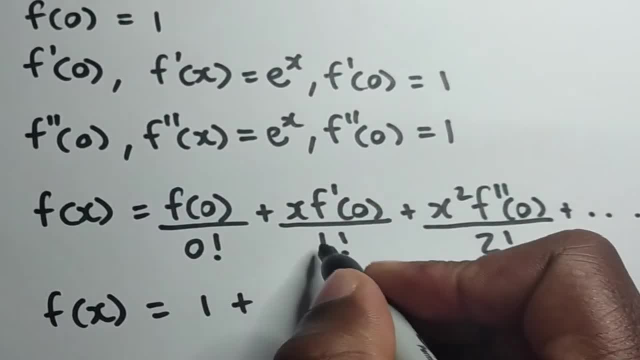 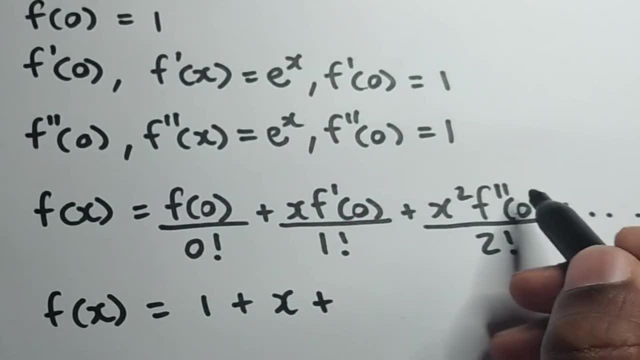 And that was one also. So one times x that will remain x over one factorial, which is one. So x over one is the same thing as x plus x squared times the result that we've got when we sub zero into the second differential of f of x. 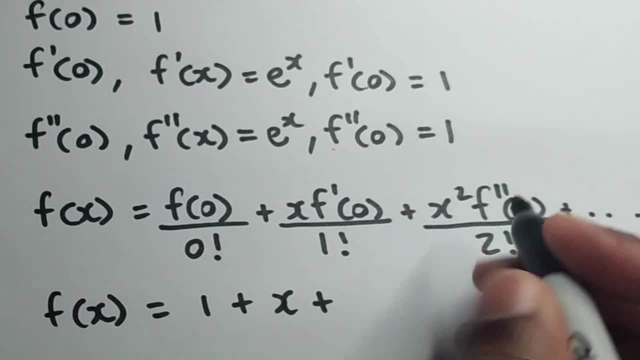 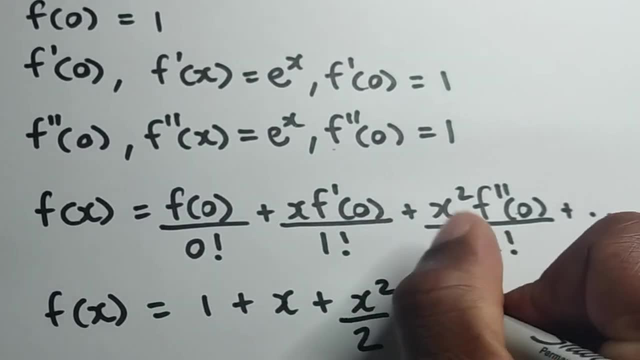 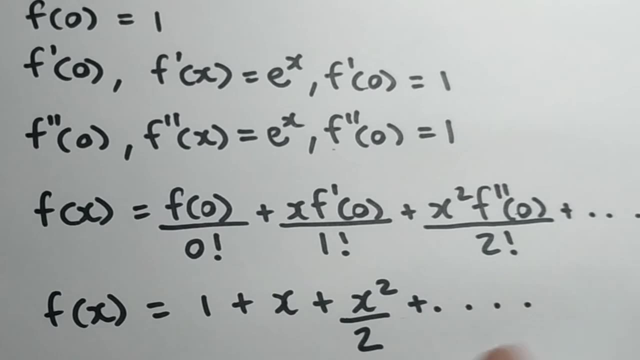 And that result was one also. So we'll have one times x squared over two factorial, and two factorial is two, All right, And this thing will continue. So this will be your answer: Are all Solution for this particular question? All right? 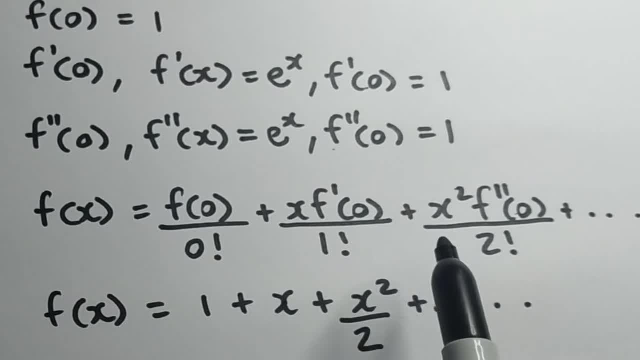 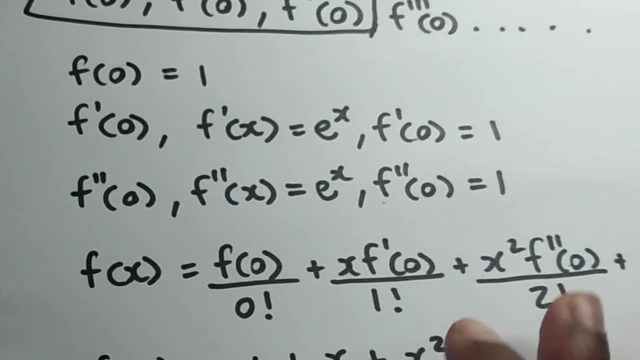 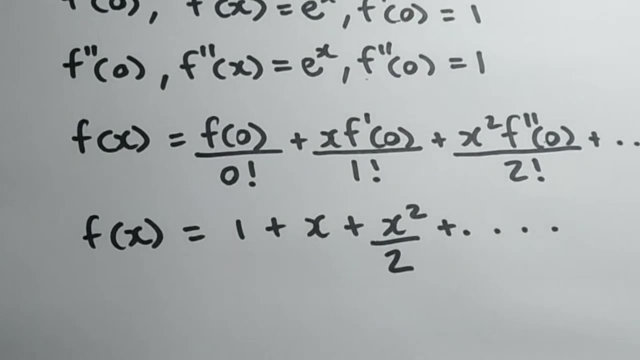 So this is how we would write Maclaurin series expansion for the f of x for the f of x function that was given in this particular question. All right, So f of x is equal to e to the x. All right, So this would be the how you write Maclaurin series expansion for this particular function. 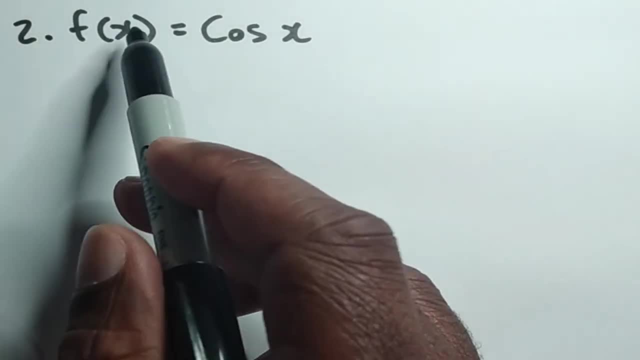 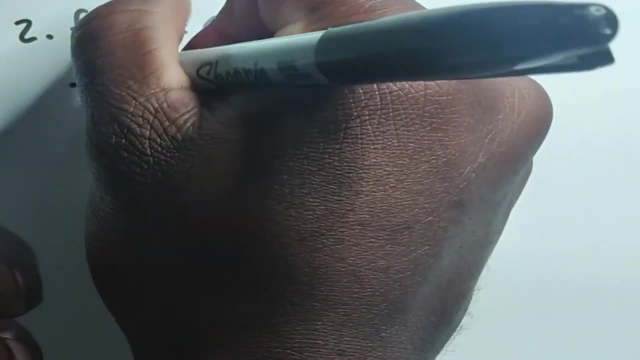 All right. Now let's look at another example. What if we had? f of x is equal to cos x, All right, So again, we want to find the things that we want to find. We are going to outline here. Want to find f of zero. 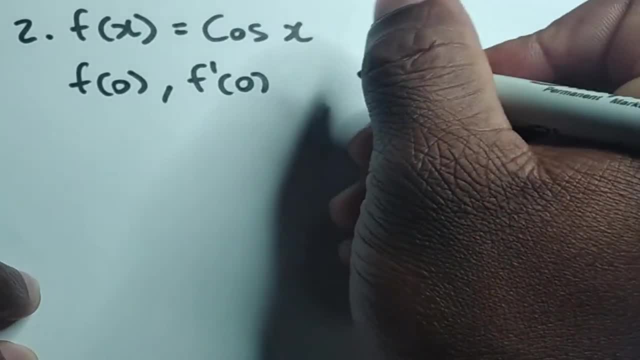 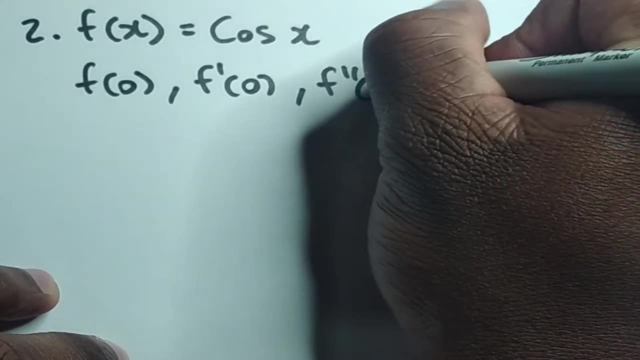 Want to find the result that we'll obtain when we sub zero into the first differential of f of x, And we also want to find the result that we'll obtain when we sub zero into the second differential of f of x. All right, And again, I'm only going to do three iterations. 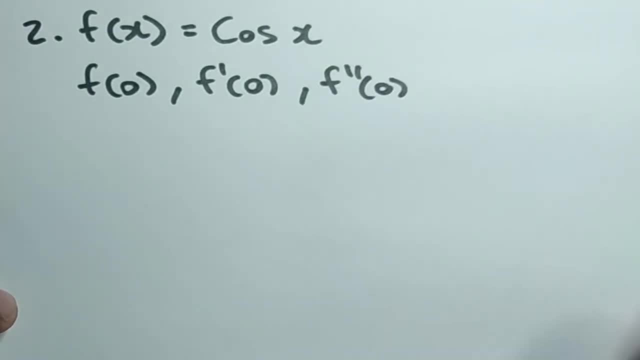 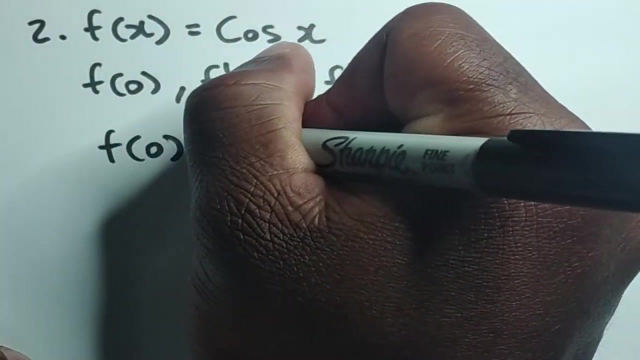 So we can get through this video In a timely manner. All right, So this will give you a basic idea, even if you are required to carry out more iterations. All right, So we want to find our f of zero. So f of zero. 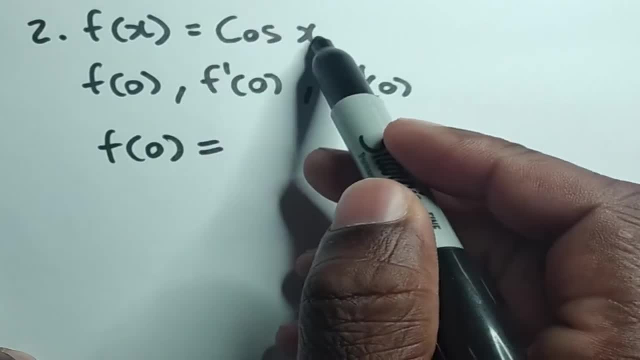 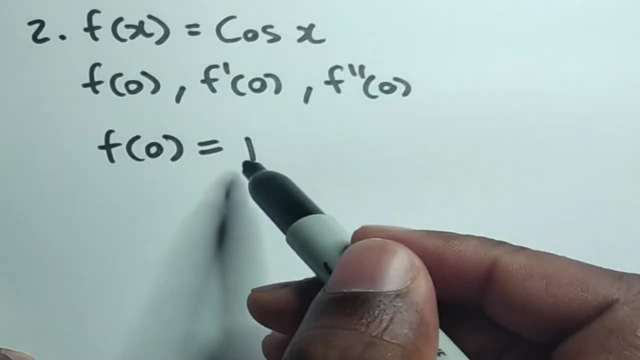 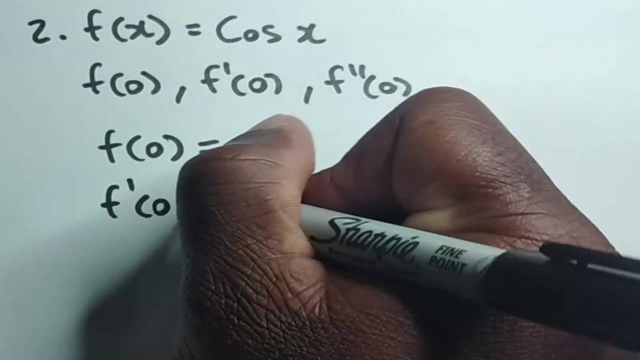 Now, if you should substitute zero in this thing, cos of zero is actually one. So if you use your calculator, cos of zero, that result that you will obtain would be one. Now we want to substitute zero into the first differential of f of x. 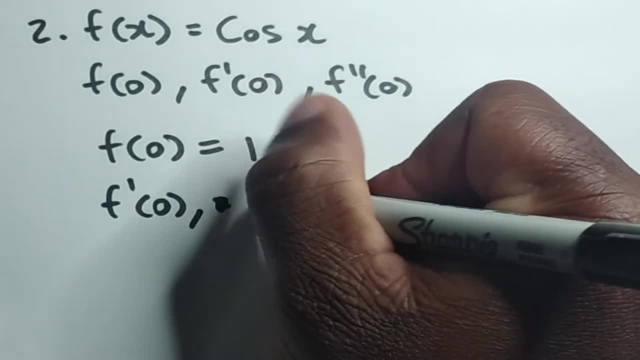 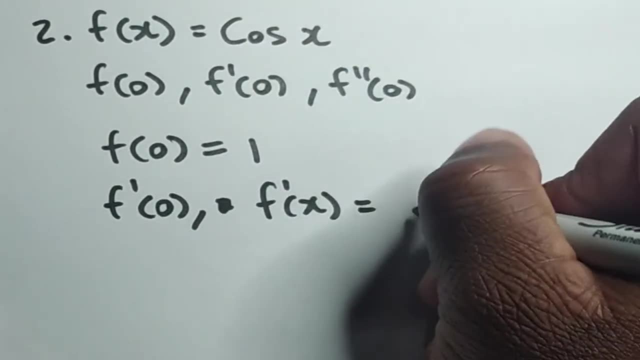 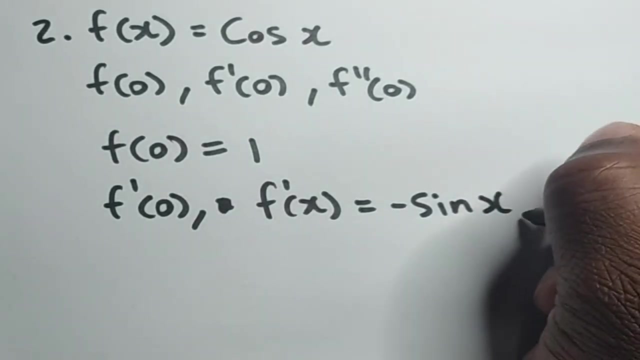 So we are required to find the first differential of f of x. So we want to find the first differential of f of x. If we should differentiate cos x, we'll obtain negative sine x. All right, So if we should substitute now zero into this function, what would we obtain? 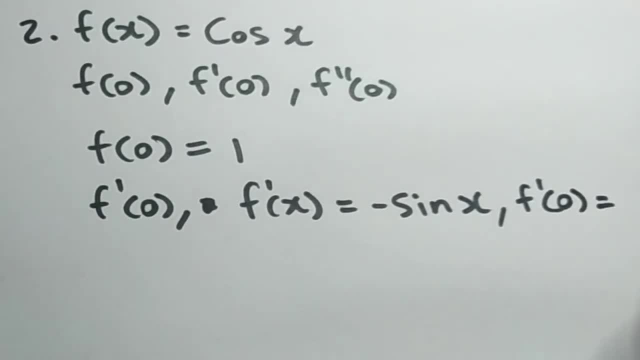 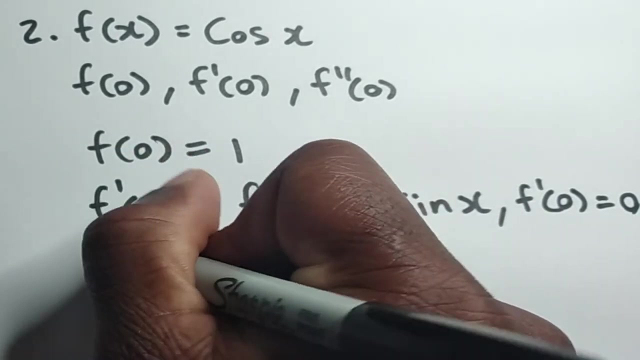 All right, All right. Sine of zero is zero. Negative zero is the same thing as zero. So the first differential: if we substitute zero into the first differential, we'll obtain zero As a result. all right, now we want to obtain the result that we'll get if we substitute zero in the second differential of f of x. 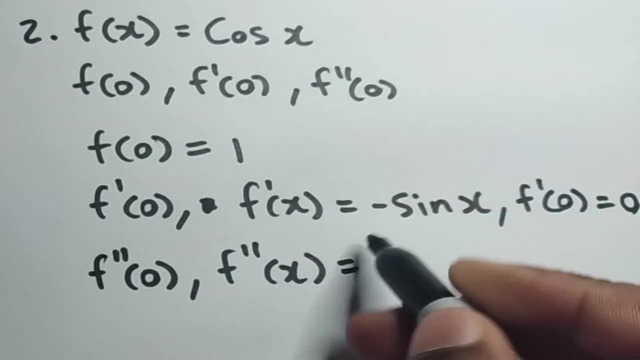 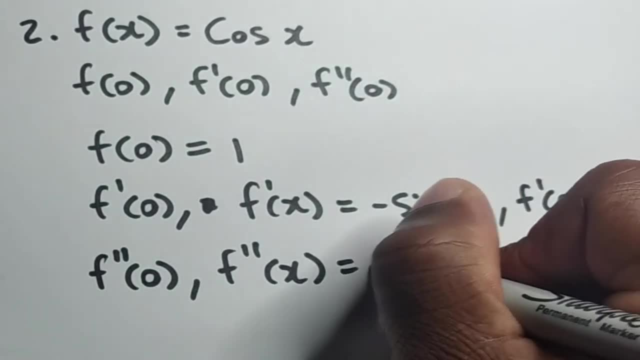 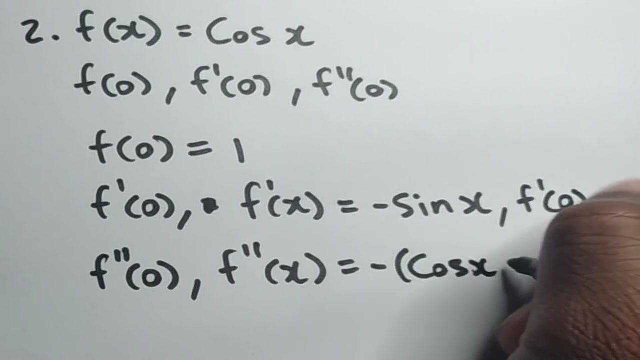 So the second differential of f of x. we are required now to differentiate the first differential to obtain the second differential. So if we differentiate sine so we can factor this negative right here. If we differentiate sine x, we'll obtain cos x. 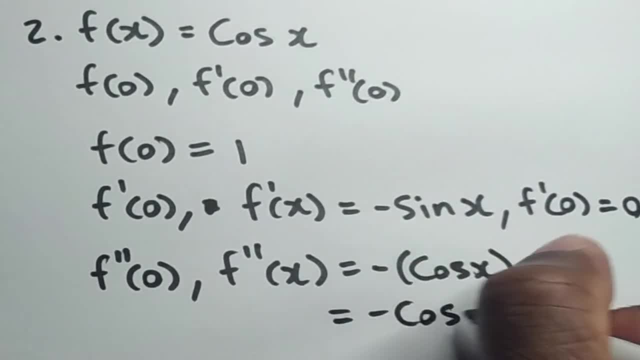 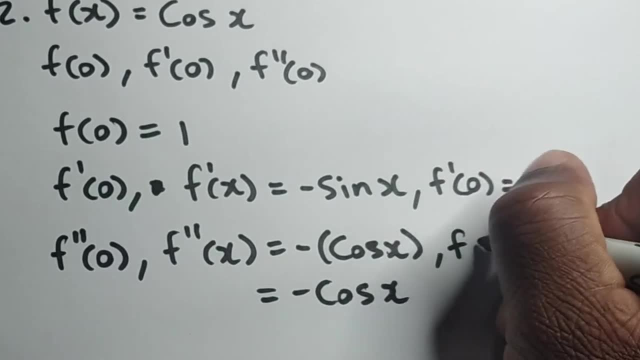 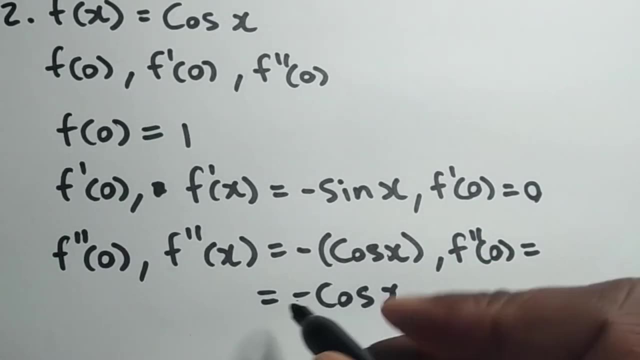 All right. So this thing is the same thing as negative cos x. All right, And if we should substitute zero into this function, that would have obtained: And again, cos of zero is one And we'll have a negative there, So we'll have negative cos of zero. 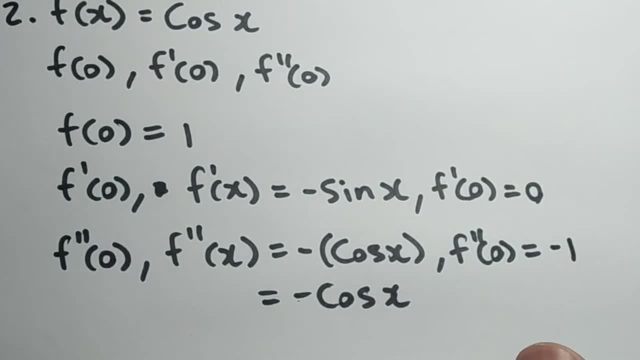 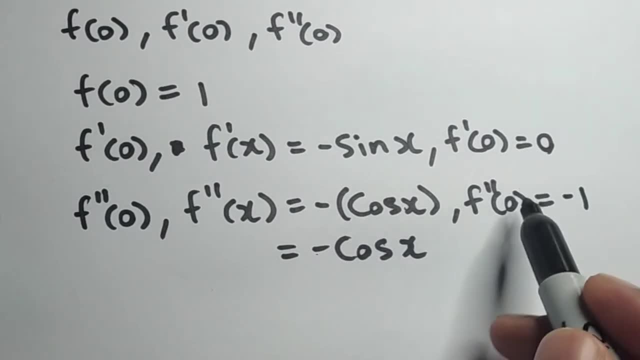 So that will give us negative one. So we'll obtain negative one there. So the result that we would have obtained, as it relates to this thing, would have been negative one. So if we substitute zero into the second differential of f of x, then we'll obtain negative one. 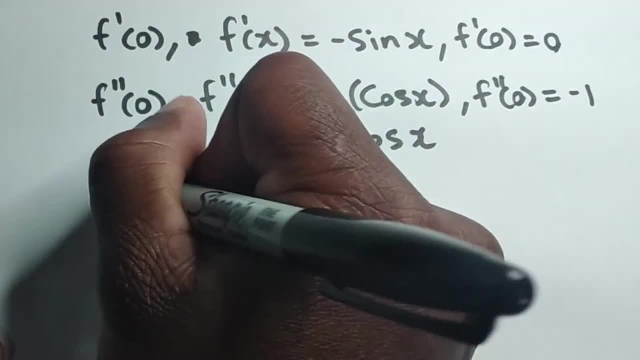 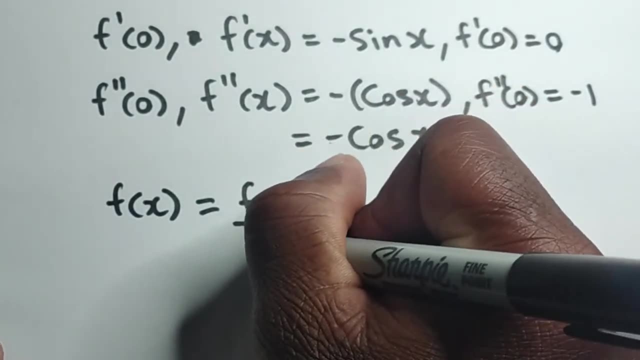 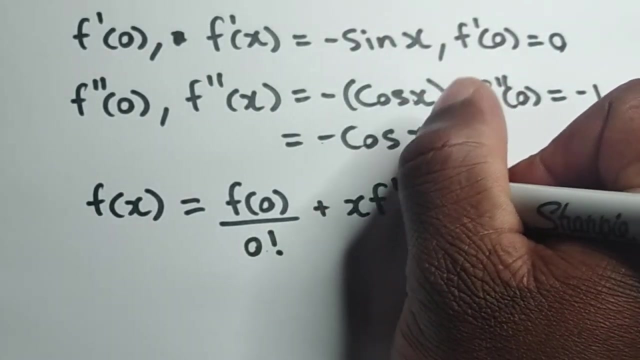 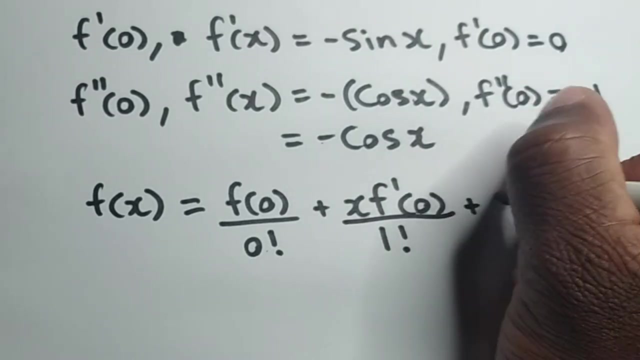 Now we want to recall the Maclaurin series formula where f of x is equal to f of zero, negative one Negative one over zero factorial plus x times the result that we get when we substitute zero into the first differential of f of x over one factorial, plus x squared times the result that we'll get when we substitute zero into the second differential of f of x, all right over two factorial. 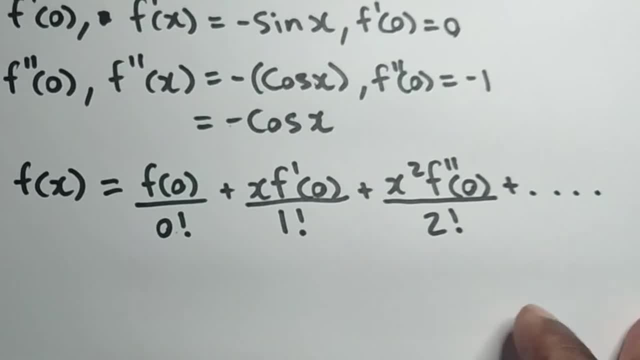 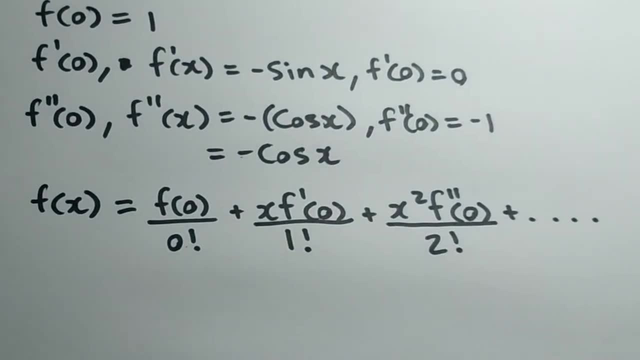 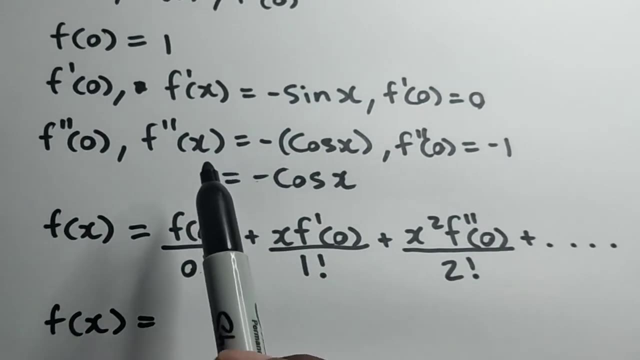 And again, we can do many iterations of this thing. All right, So how do we plug in these values now? Again, we'll do the same thing as the previous example. So we have our f of x. what was the value that we got for f of zero? 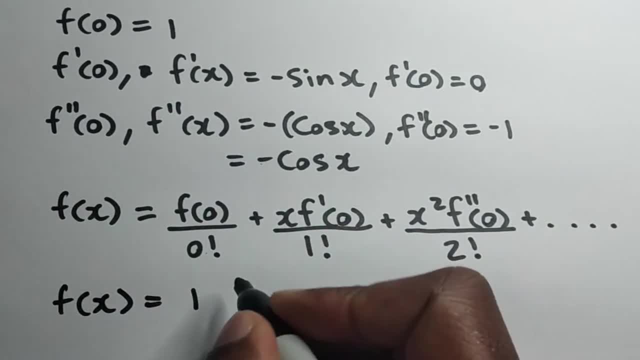 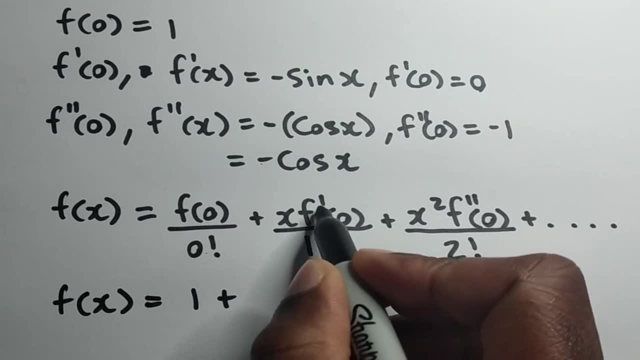 F of zero is one, So we have one over zero factorial, which is one, So one over one is one again. Now we'll have what x times the result that we got when we substitute zero into the first differential of f of x. 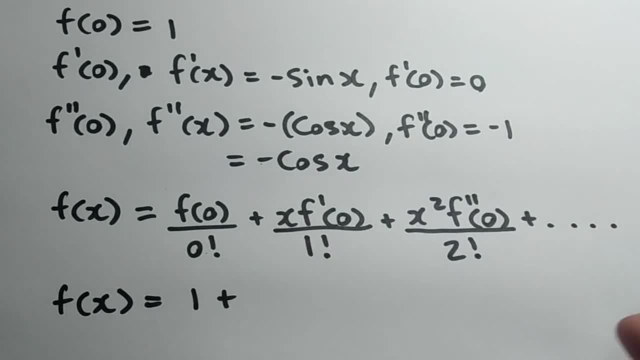 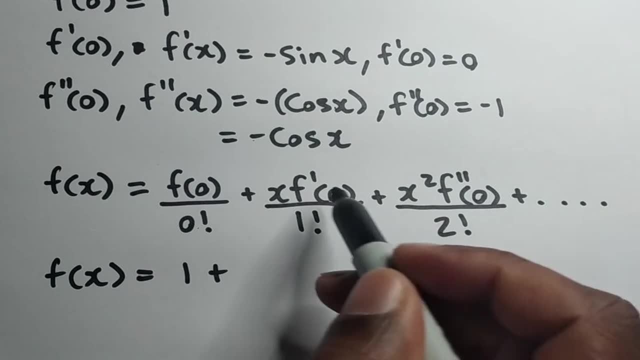 And that result was zero. So zero times x, that's the same thing as zero. All right, All right, So. so we don't even need to look at this one factorial here. So that will end up with zero over one. All right. 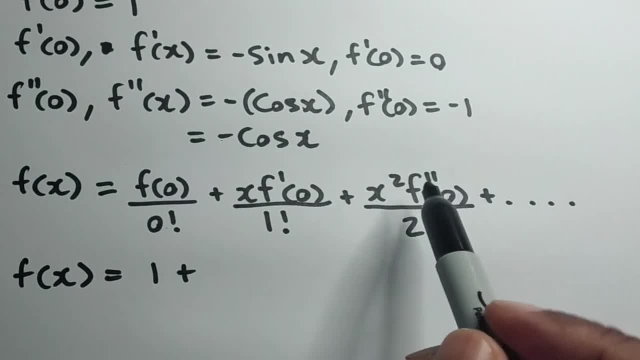 And zero divided by anything is zero. What will we obtain? also, We have what x squared times the result that we'll get when we differentiate, when we solve zero into the second differential of f of x, And when we did that, we got negative. 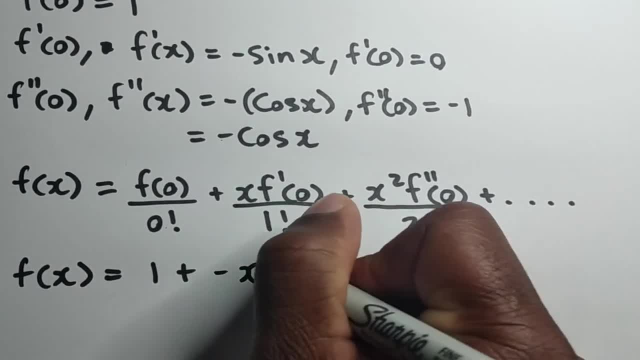 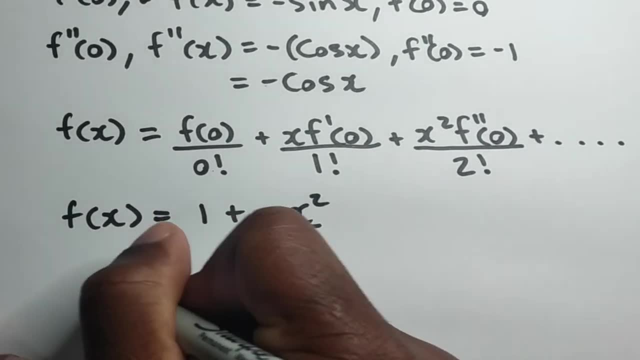 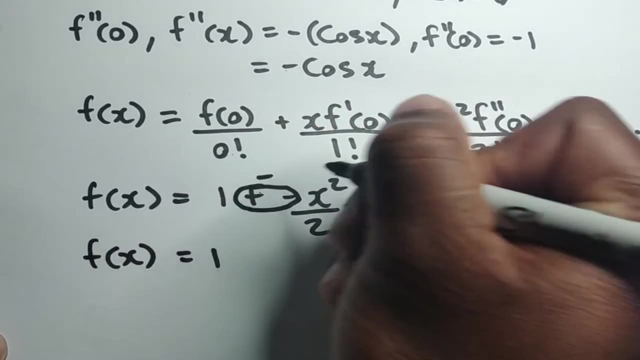 One. So we'll obtain negative x squared over two factorial, which is two. All right, We can write this in a simpler form. So in this case, f of x is equal to one. This positive and a negative sign will give me a negative. 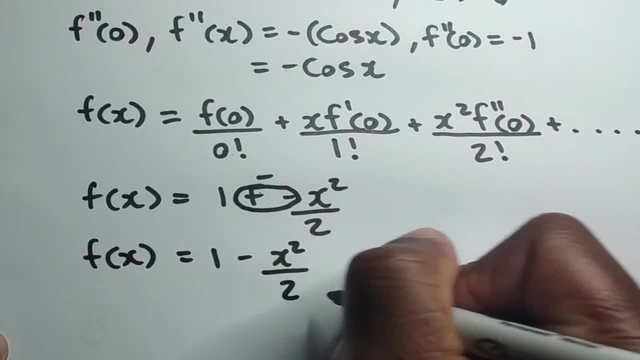 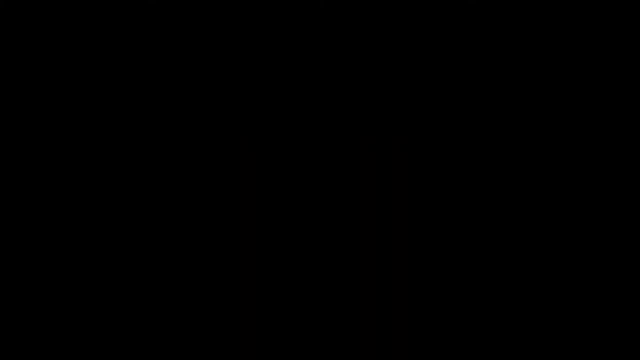 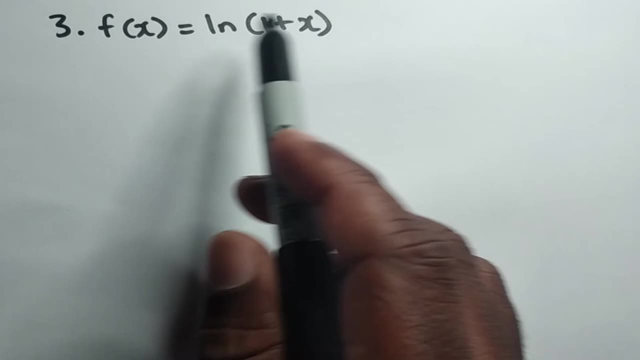 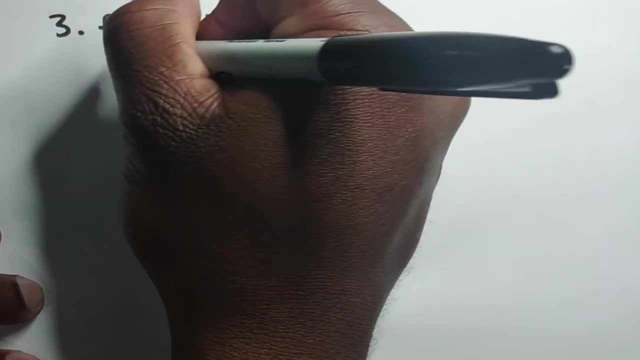 So this is one minus x squared over two. Now let's look at how we can write Maclaurin series expansion. for this particular function, f of x is equal to ln of one plus x. All right, So again we know that we're going to need what. 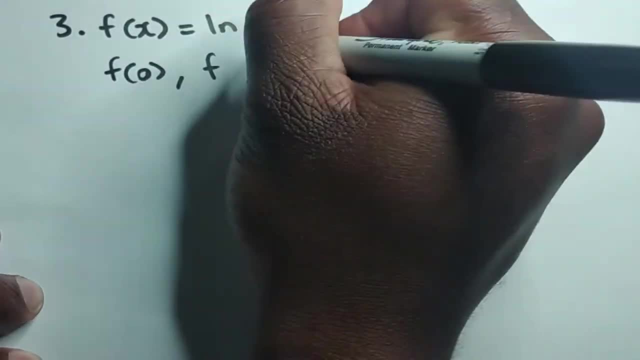 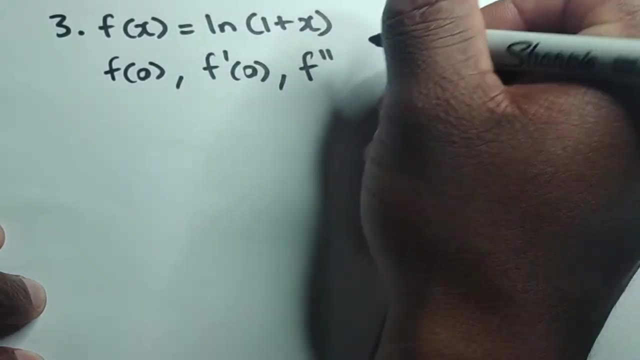 We're going to need the result f of zero. We're also going to need the result that we'll obtain if we solve zero into the first differential of f of x. And we're also going to need the result that we'll obtain if we solve zero. 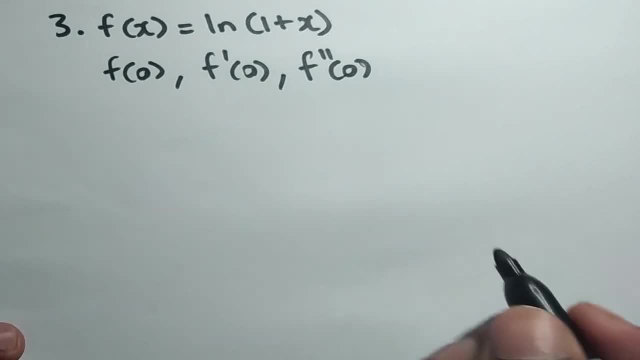 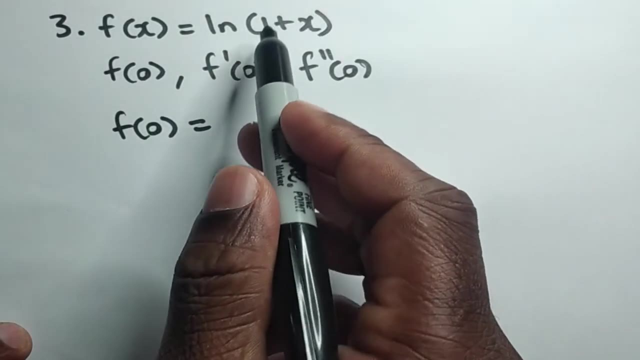 into the second differential of f of x. All right, So let's first find our f of zero. Now, if we should substitute zero in this function right here, we'll end up with ln one. All right, Because one plus zero is one. 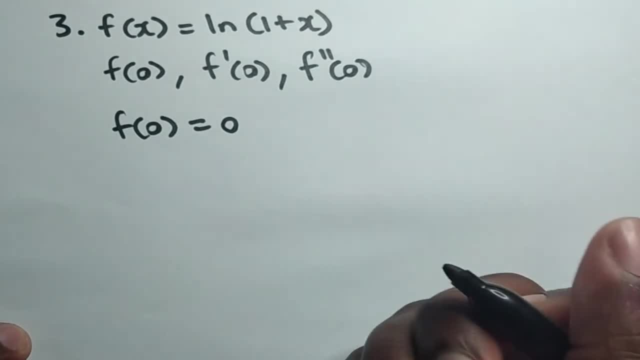 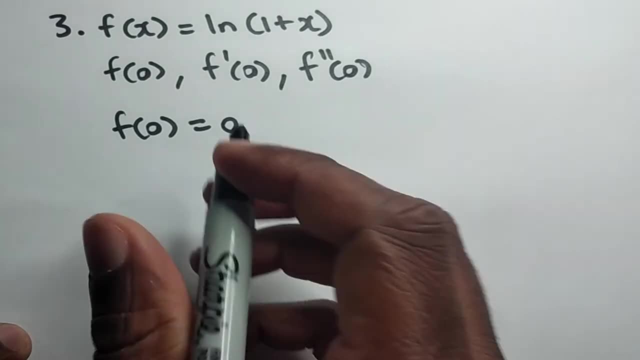 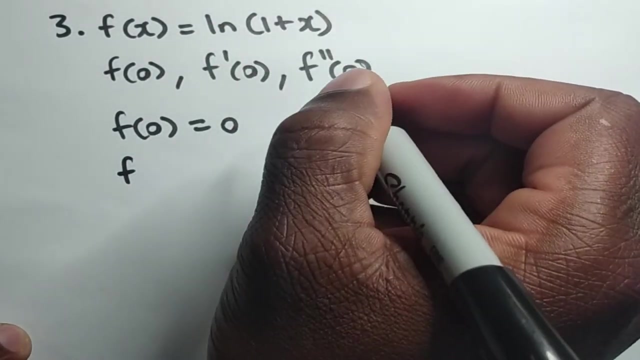 So ln of one will give us a zero right here, And you can always test these results in your calculator. All right, You can always check that out. So now we want to find what In order to Substitute zero in the first differential of f of x. 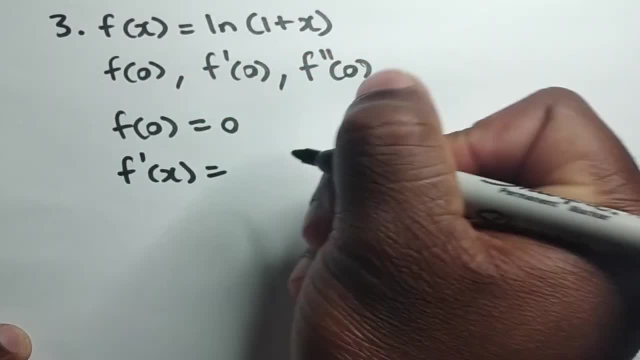 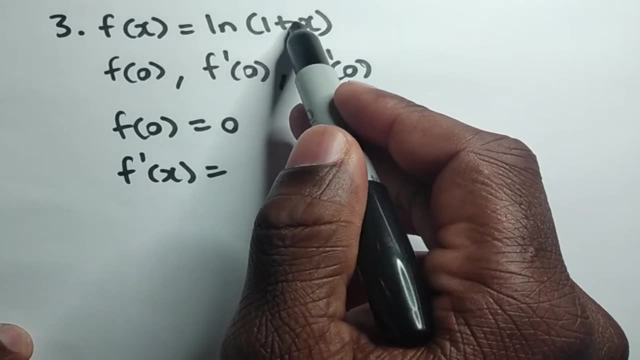 We must first know the first differential of f of x. All right, So if we differentiate an ln function, ln of whatever will differentiate that. So we have ln of one plus x will differentiate the one plus x And that will give us a one. 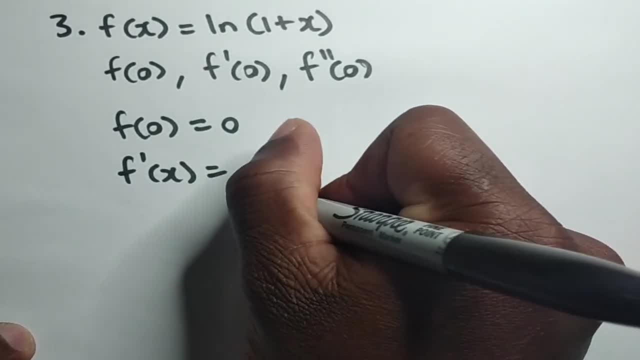 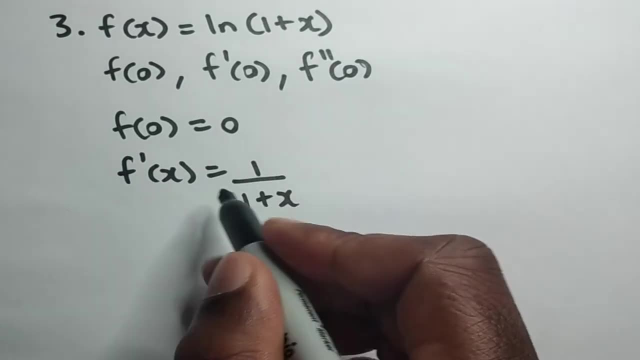 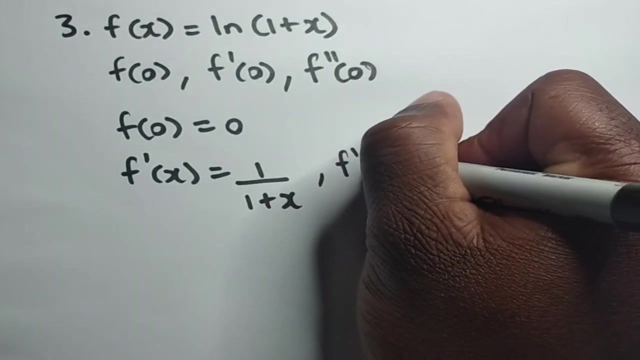 Then we'll put that result over the function itself. All right, So that's how you treat with the differential of an ln function. So This will give us the first differential, will give us one over one plus x. If we should substitute zero in this thing, what will we get? 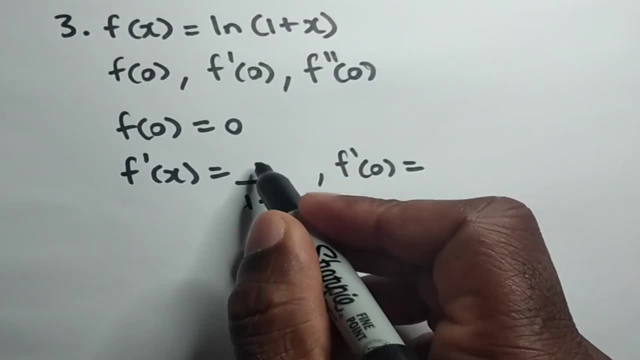 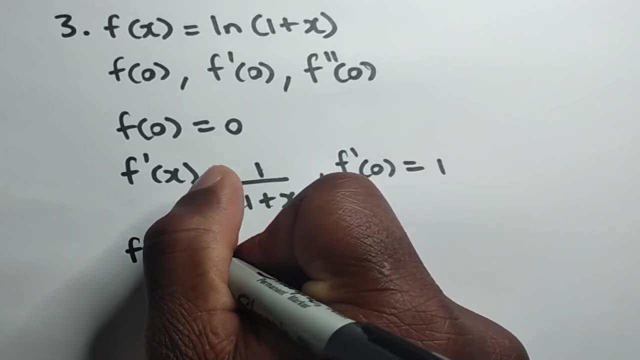 All right, One over one plus zero. This will give us one, So we'll have one over one And that's one. All right, And the final iteration, for the sake of this video, we'll find the second differential of this thing. 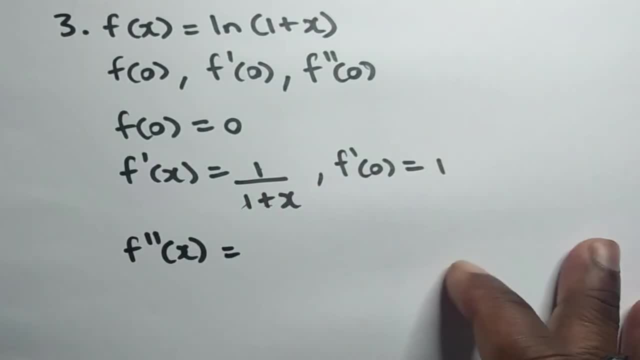 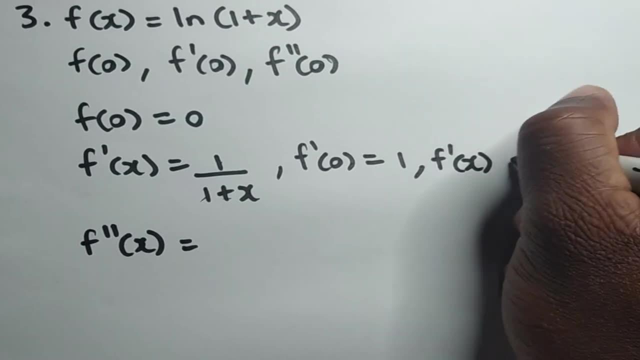 Now what we could do. All right, We can rewrite This function, All right. So first, differential of x can also be written as we can bring up the denominator. So we can bring this thing up in the top and it will become one plus x to the power of negative one. 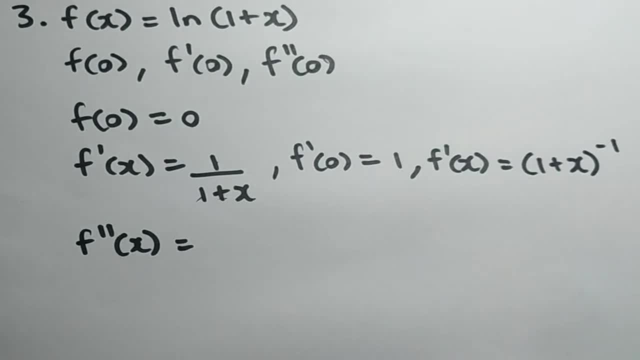 All right, So that's the same thing. So we can do that. So this is easier to differentiate. Of course, we could differentiate this thing using the quotient rule, But I guess you choose how you want to do it, All right. 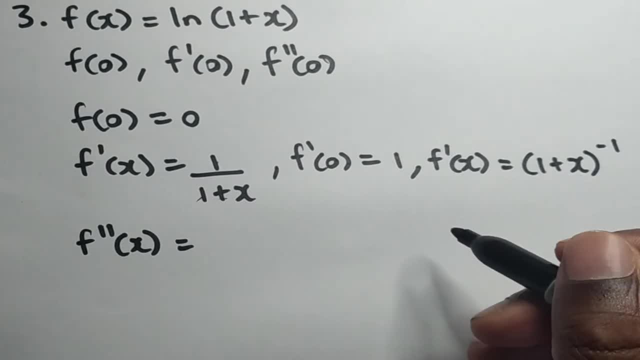 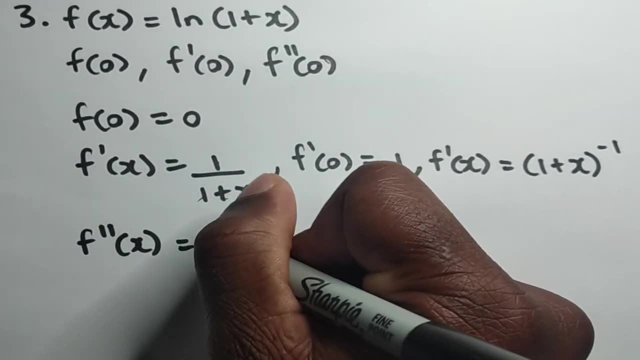 But I prefer to do it like this. However, anyways, work anyhow, All right. So we're going to use a chain rule to differentiate this thing. So we're going to multiply the bracket by four, So we have negative one times what we have in the bracket. 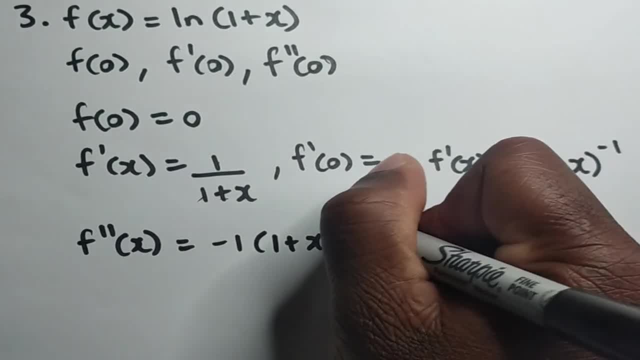 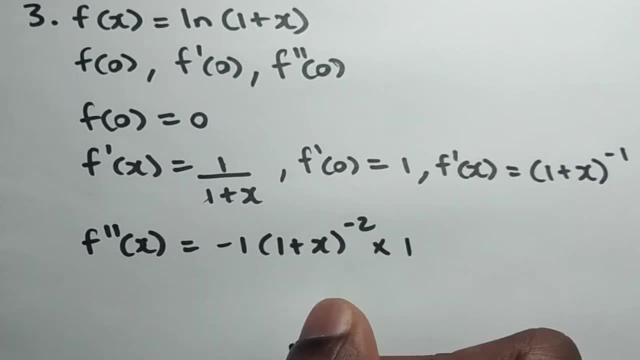 One plus x, Then we'll minus one from the power, We'll have negative two. Then we'll multiply this thing by the differential of the bracket, which is one. All right, So this is the same thing as negative one times a bracket. 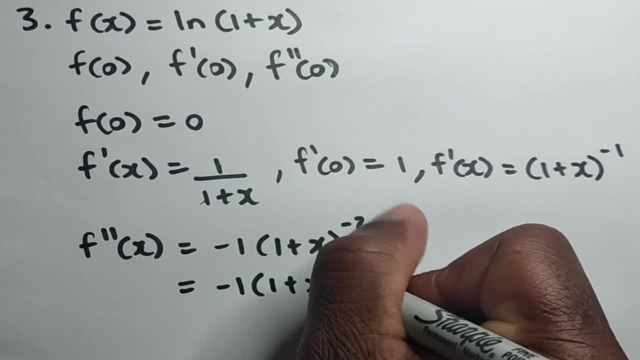 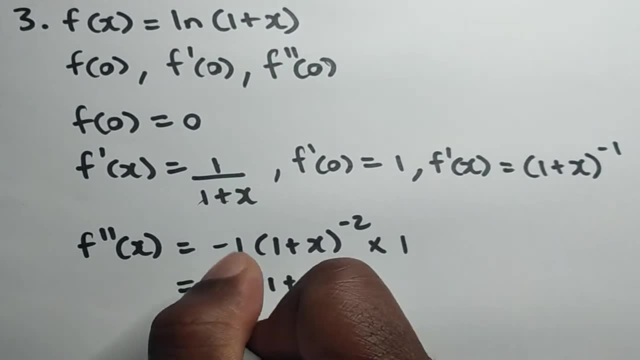 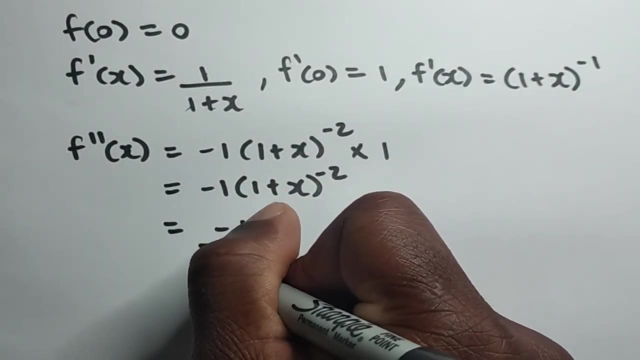 All right, All right Times the bracket, which is one plus x, to the power of negative two. All right, Because one times anything don't change the value of the thing. We can also rewrite this thing as negative one. We can bring this bracket down in the denominator. 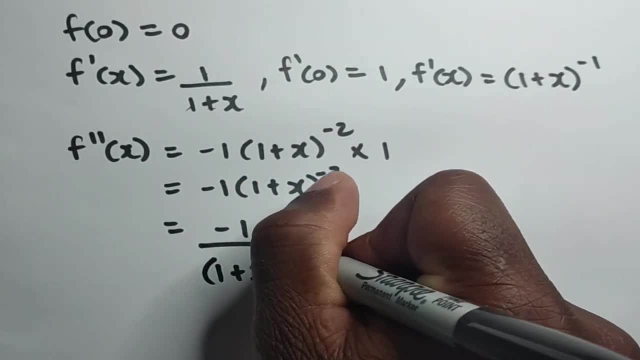 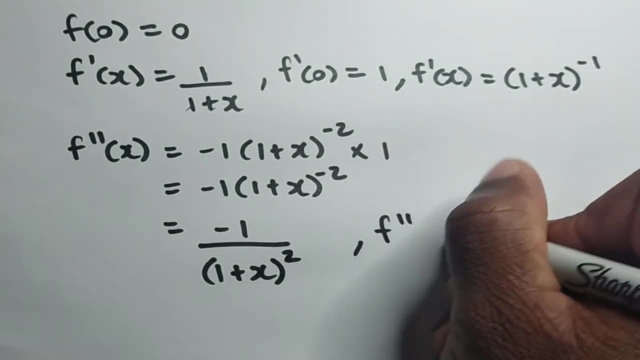 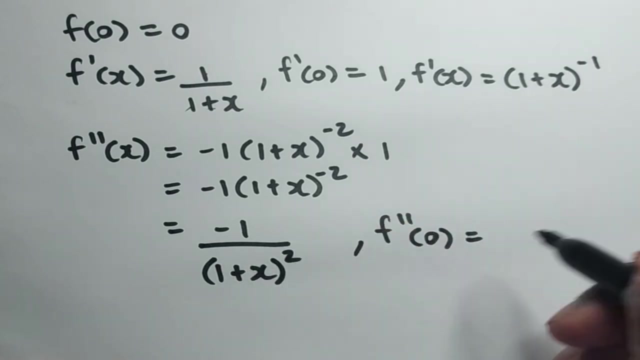 It's the same thing as one plus x in bracket raised to the power of two. All right, So we can do that. Now we want to find what the result that we'll obtain when we sub zero into this, Into the second derivative, which is negative, one over one plus x, all squared. 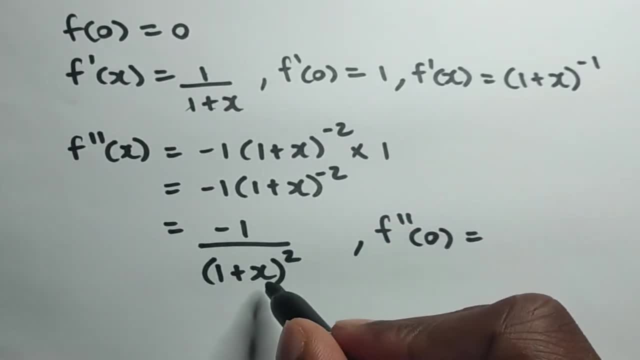 All right. So if we should substitute zero in this thing, we'll get one plus zero, So we'll only be left with one in the bracket. One squared is one, So we'll end up with negative one over one which is negative one. 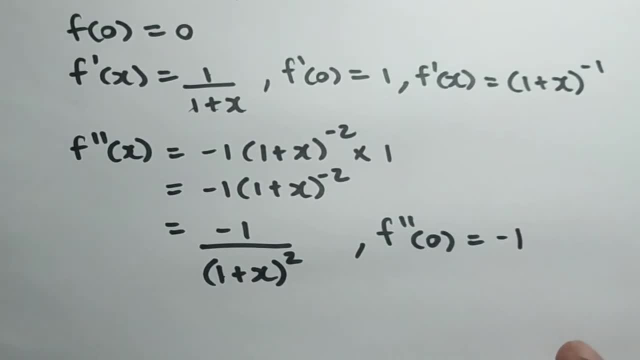 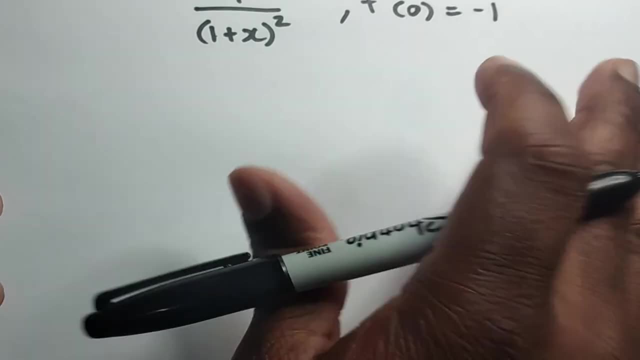 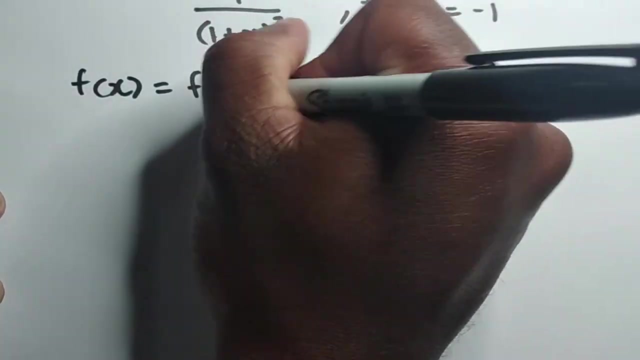 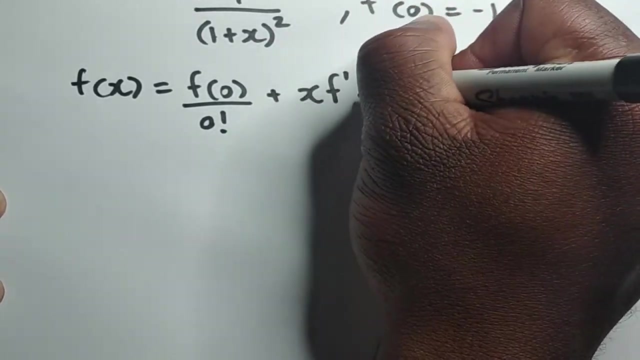 All right. So what we want to do now is to plug in these values into the Maclaurin series formula. All right, So recall the formula. And the formula is what F of x is equal to f of zero over zero, factorial plus x times the first differential. 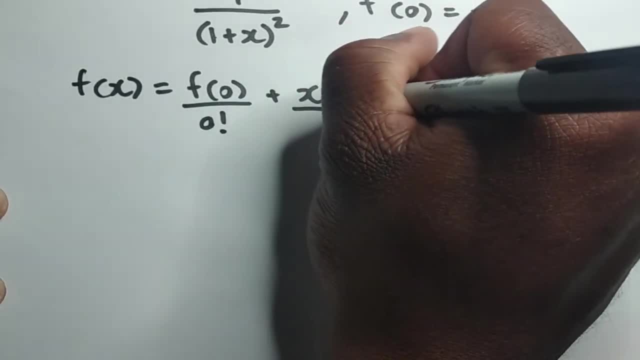 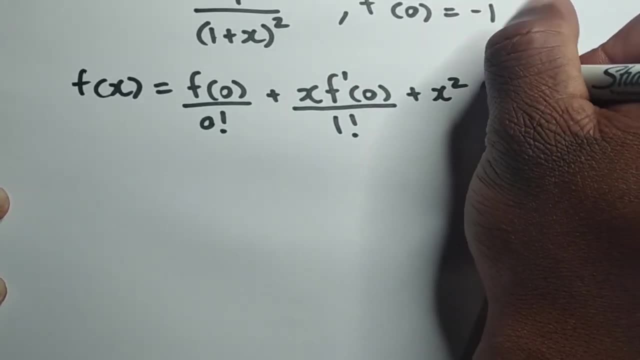 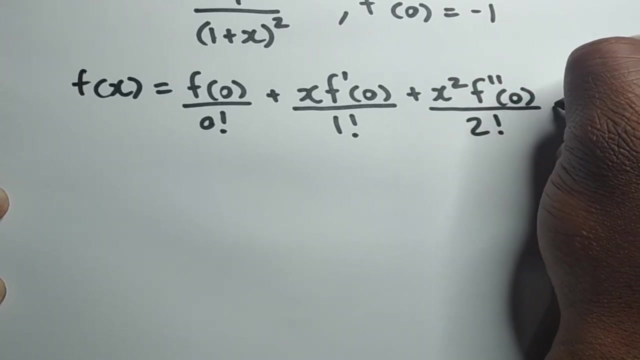 The result that we'll get when we substitute zero into the first differential of f of x over one factorial, plus x squared times the result that we'll obtain when we sub zero into the second differential of f of x. All right, So we'll get negative, one over one, plus x over two factorial. 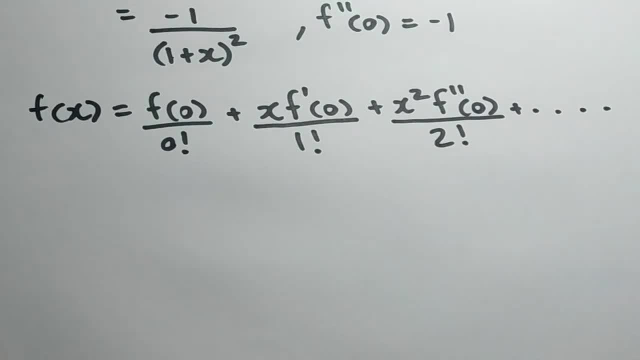 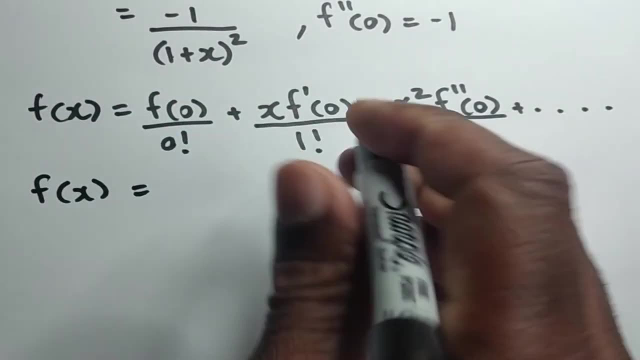 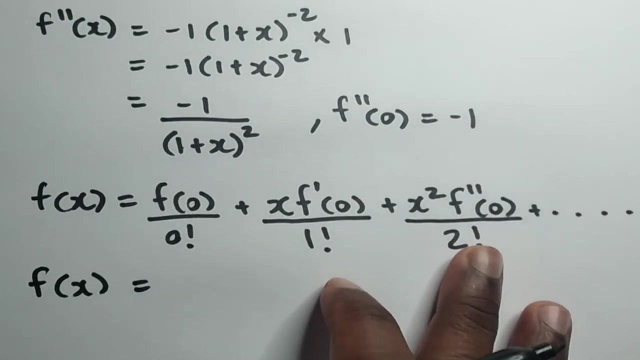 And again this thing continues. We can have many iterations of this thing. All right, So we're going to plug in the values that we've got now. So f of x is equal to what was our f of zero. Well, f of zero was actually zero. 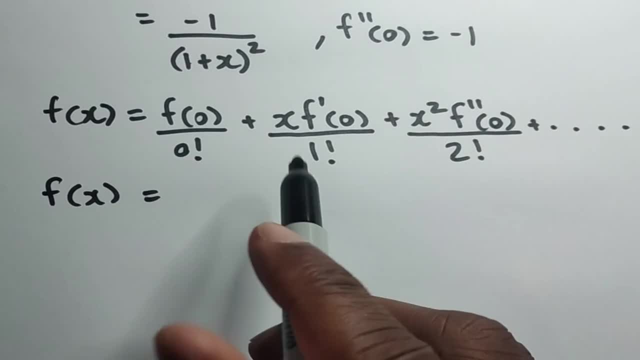 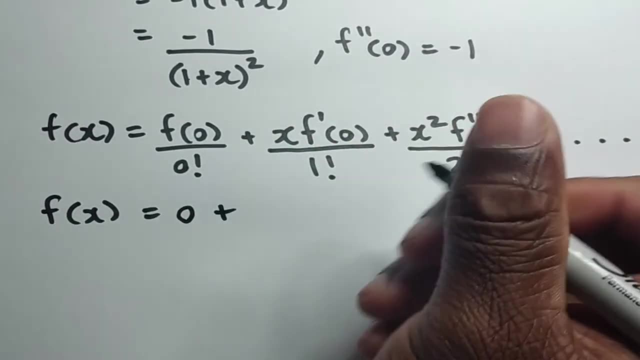 All right, So we'll have zero over one. So zero divided by anything is zero, So we don't need to, But right here, in fact, we can write it. So we'll have zero plus. let's see what we'll have here. 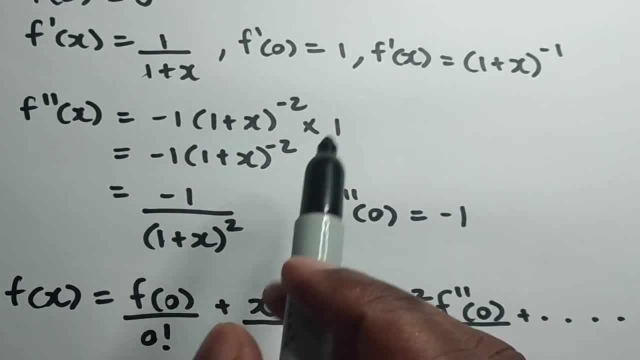 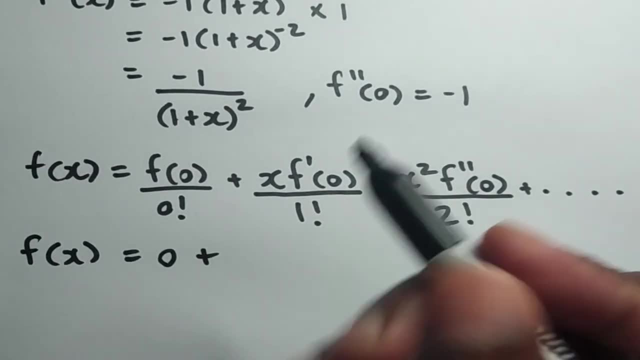 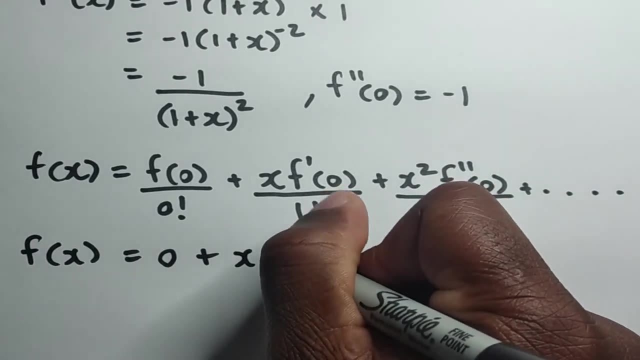 No. What was the result that we got when we substitute zero into the first differential of f of x? That was one, So we can have x times one here, which is x over one factorial. So x over one is same thing as x plus here. 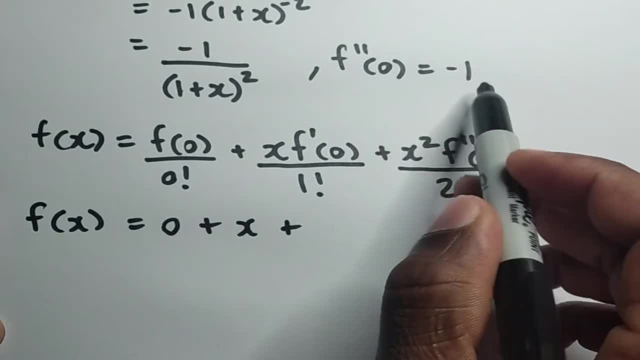 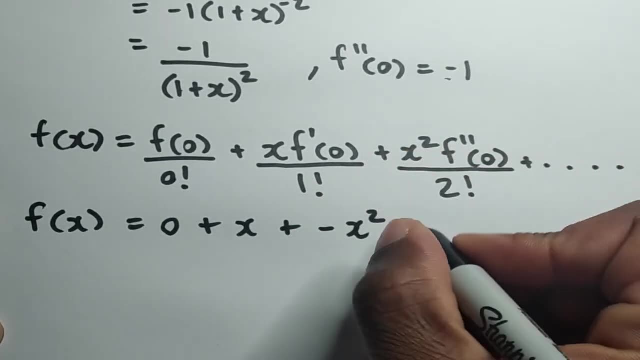 No, The result that we got when we substitute zero into the second differential, The result that we got when we substitute zero into the second differential, was what Negative one? All right, So we'll have negative x squared over two factorial, which is two. 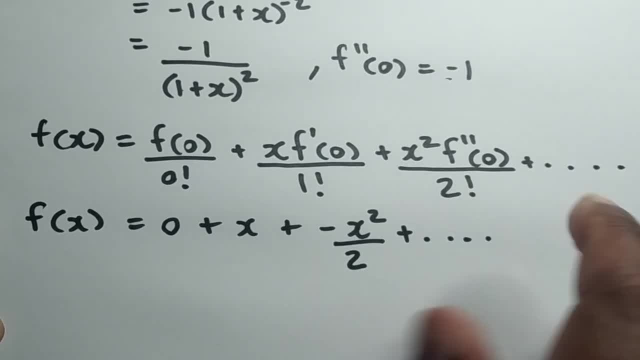 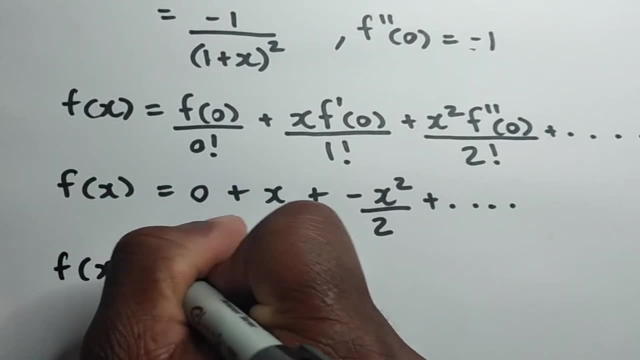 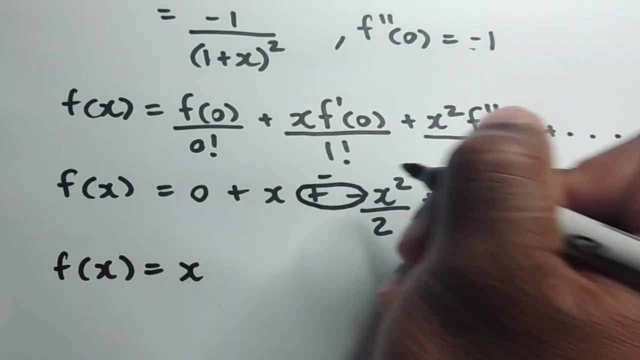 All right, And again, we could have had more iterations of this thing. So that's where we'll stop. So f of x is equal to don't have to rewrite that zero. So x again have a positive and a negative, We get a negative result. 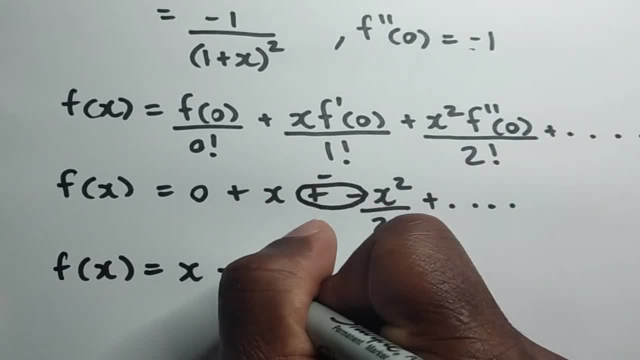 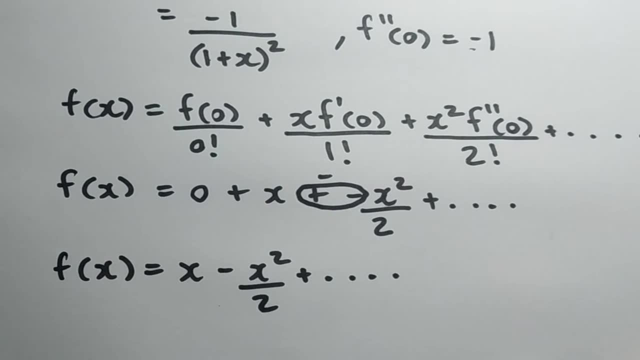 So x minus x squared over two. We could have had more iterations of this thing, All right, So this would be the result for this particular function. So this is how we would write Maclaurin series expansion for this particular function. And here we have the final example that we'll be looking at today. 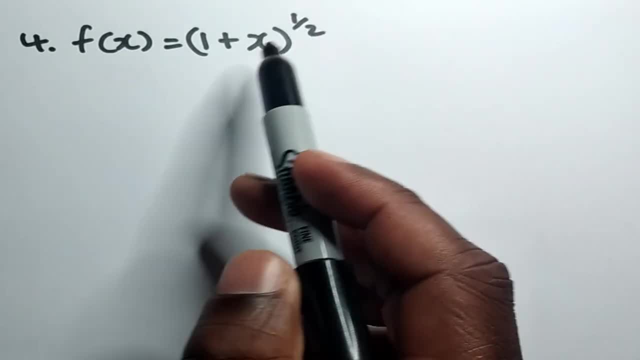 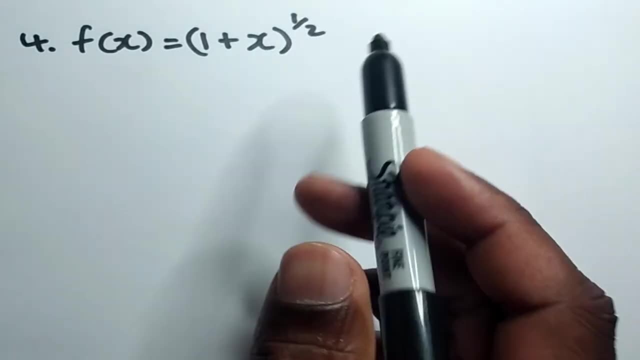 So we are going to look at how we write Maclaurin series. expansion for the function f of x is equal to zero. So we are going to look at how we write Maclaurin series. expansion for the function f of x is equal to one plus x, all raised to the power of a half. 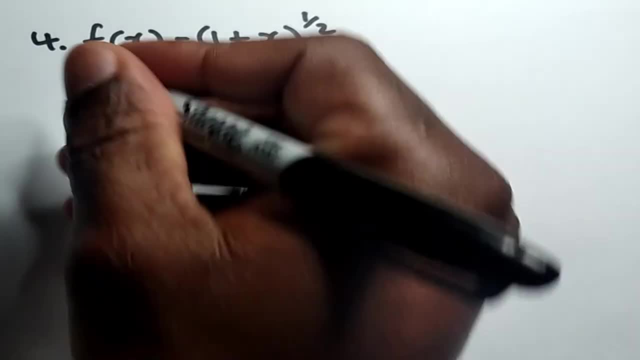 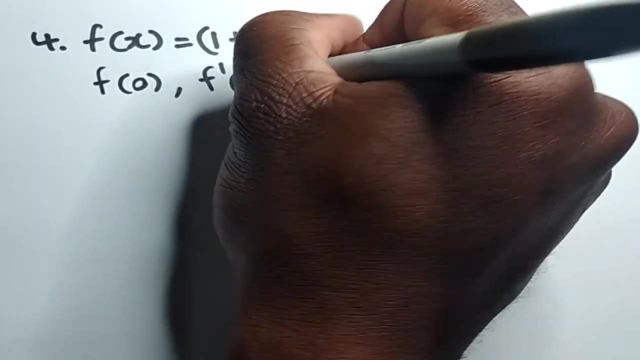 All right. So how do we do this? Again, we need to find our what We know, that we need to find f of zero. We need to obtain the result that we'll get when we substitute zero into the first differential of f of x. 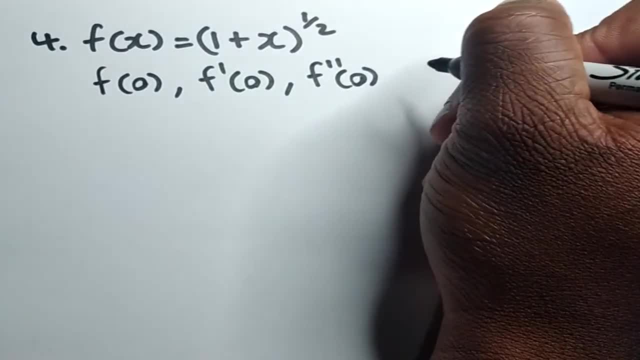 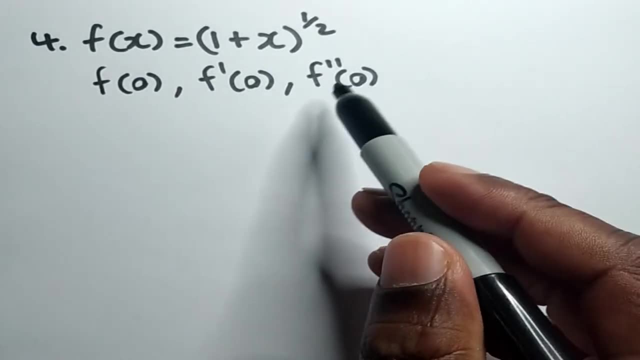 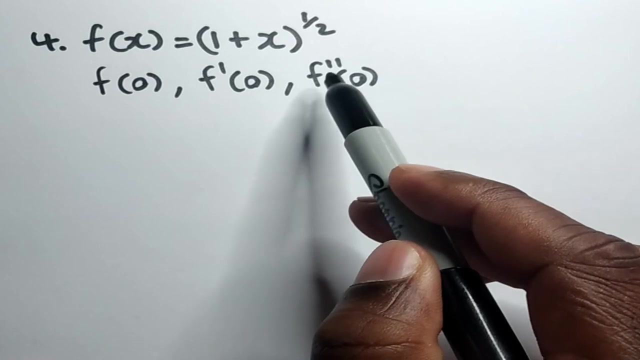 We also want to know the result that we'll obtain when we substitute zero into the second differential of f of x. And again, always bear in mind that you can have more iterations of this thing, All right. So if we wanted to do one more iteration, we'll also be required to find the result that we'll get when we substitute zero into the third differential of f of x. 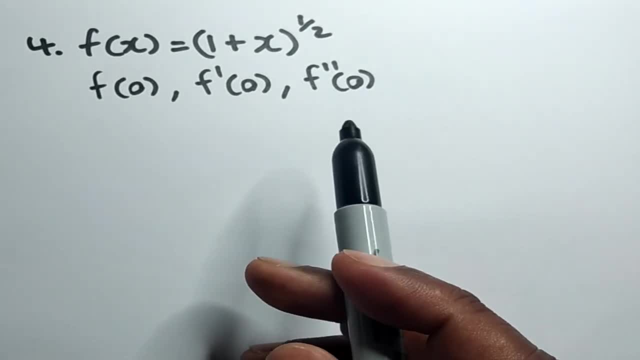 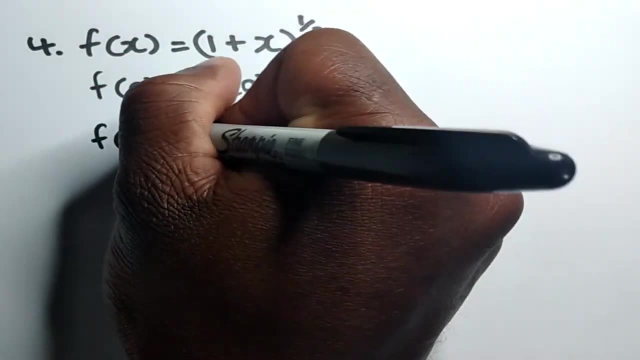 All right, So always bear that in mind. So this is the final example in this video. All right, Now let's obtain the values that we need. So f of zero If we should substitute. So a key thing to note is that f of x here. 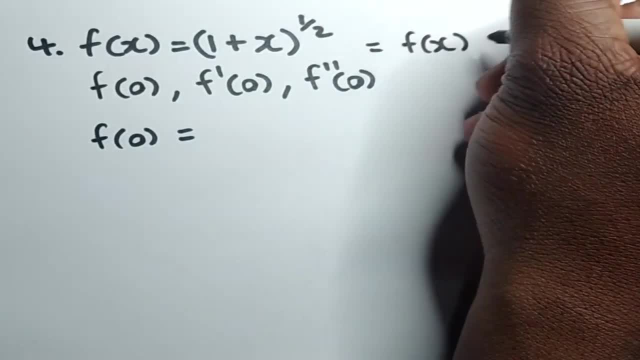 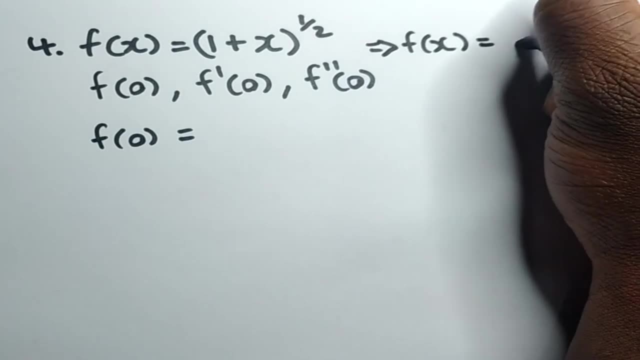 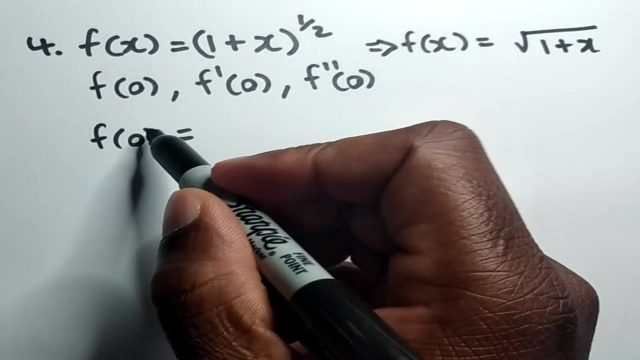 f of x is equal to. this is the same thing as one plus x. raised to the power of a half is the same thing as the square root of this entire thing right here, All right, So always bear that in mind. So f of zero. 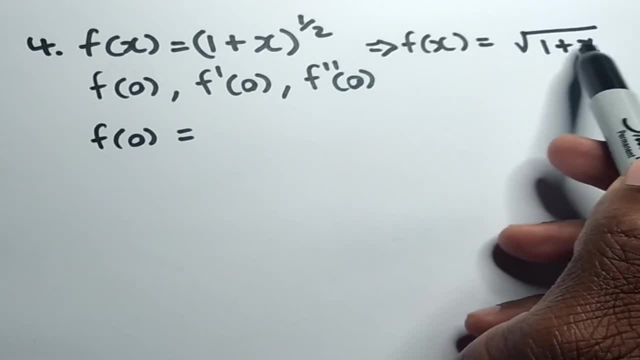 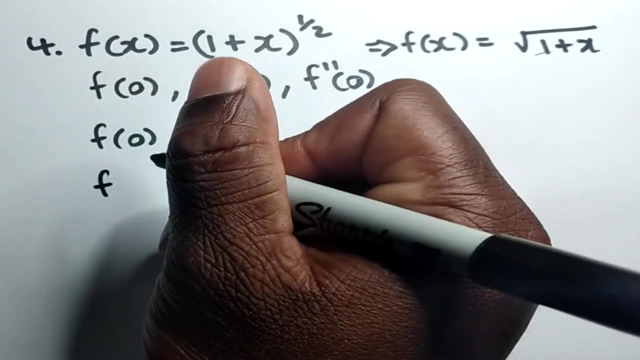 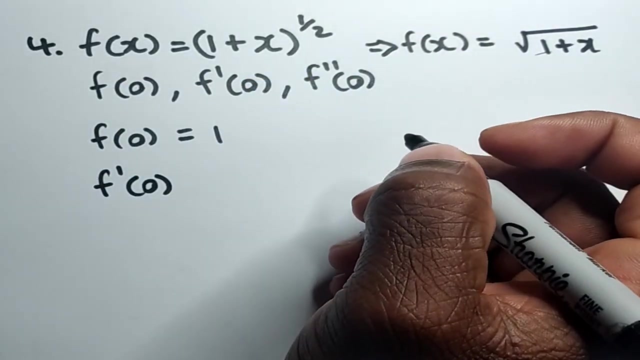 If we should substitute zero here, we'll have one plus zero. The square root of one is one, So f of zero is one. All right, Now I want to find what f the result that we'll obtain when we substitute zero into the first differential of f of x. 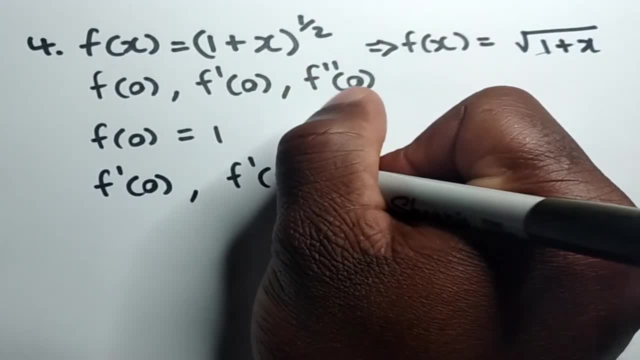 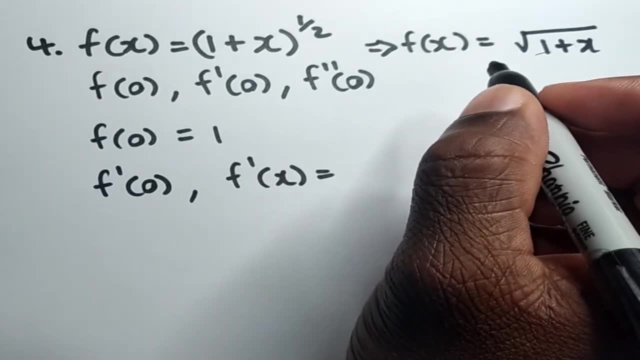 All right, So I want to find the first differential of f of x. And what is that? If we should differentiate this thing? we can differentiate this thing using the chain rule, But what would we obtain? We'll multiply the function by the power. 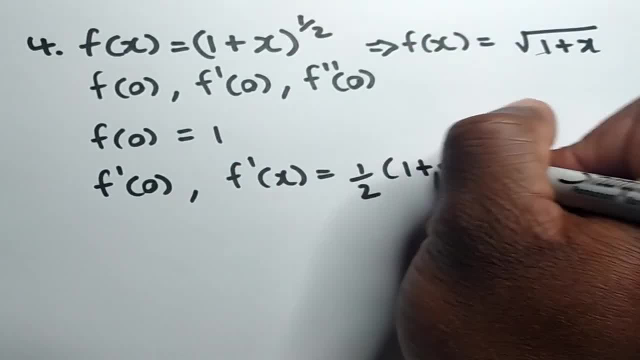 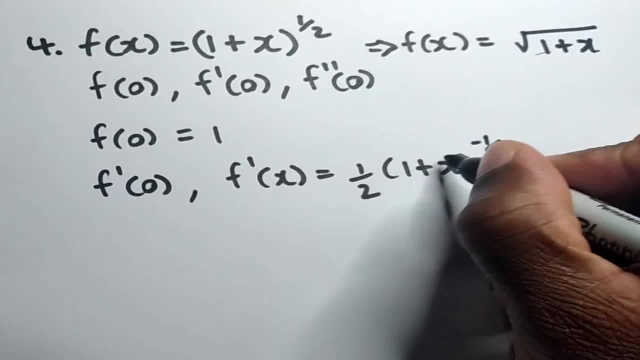 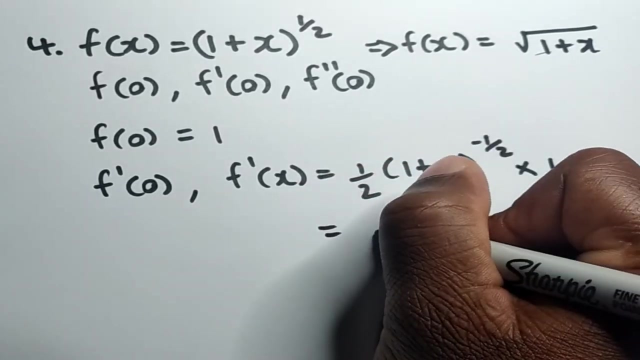 So we have a half times one plus x. We'll minus one from the power, So we'll end up with negative a half. I will multiply that by the differential of the bracket, which is one. All right, So this is the same thing as, let's see, a half times. 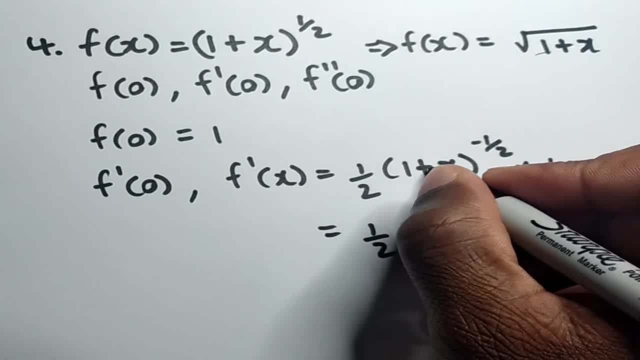 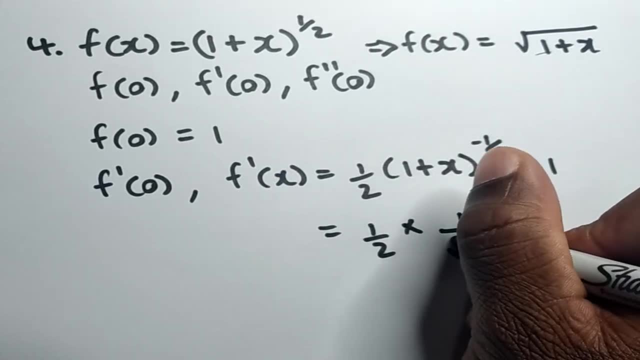 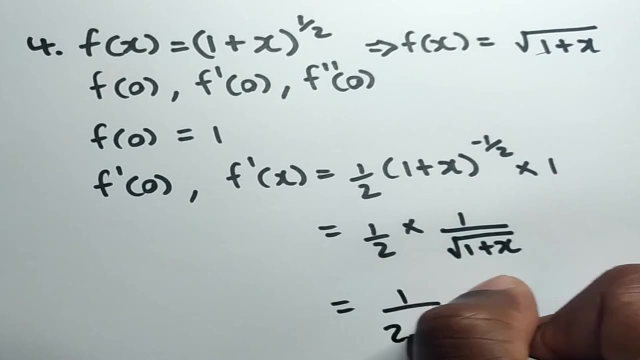 We'll have here now Let me see. We can rewrite one plus x to the power of negative a half as what? One over the square root of one plus x. All right, So this is the same thing as one over two times the square root of one plus x. out here. 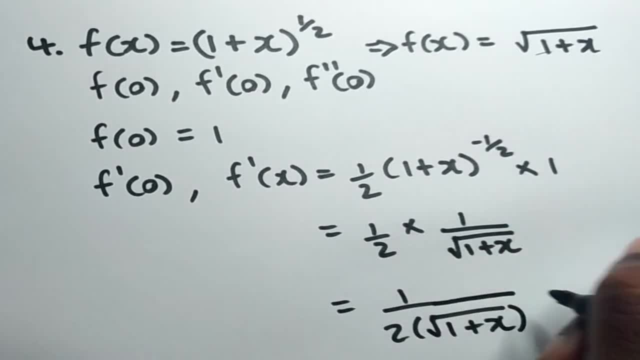 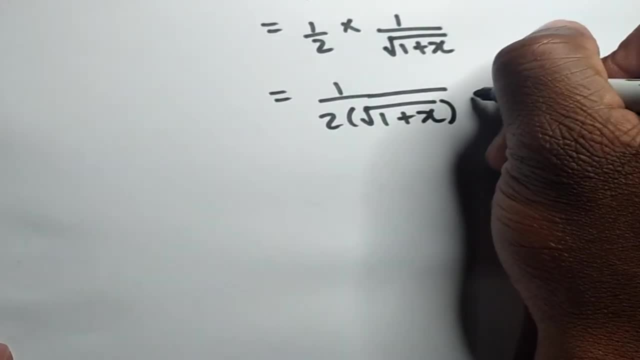 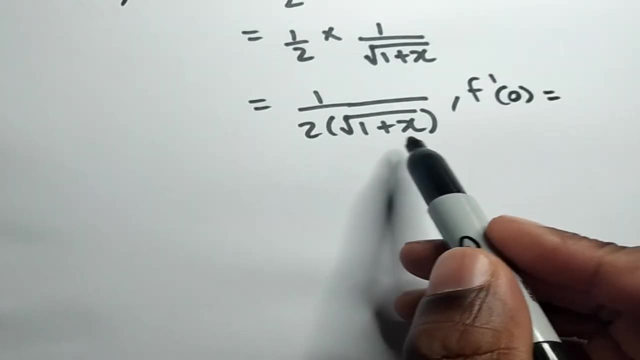 All right, So we can do that. Now, if we should substitute zero into this function that we got for the first derivative, we'll end up with one plus zero, All right, So one plus zero. So one plus zero is one. 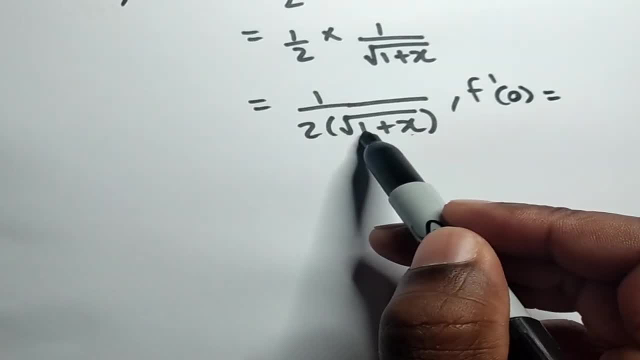 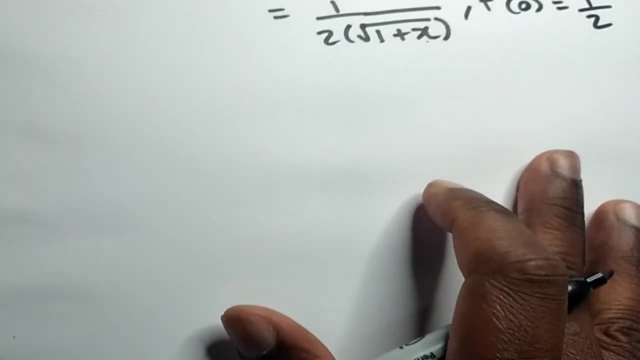 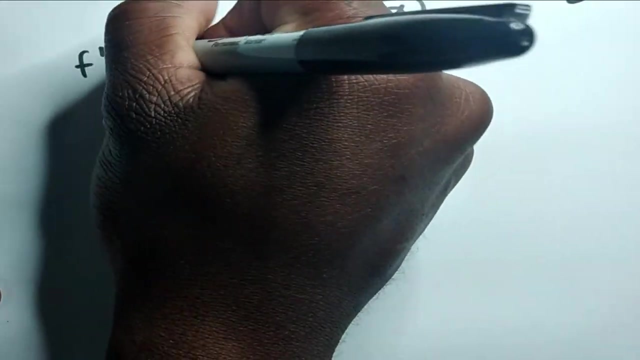 The square root of one is one. Two times one is two, So we'll end up with one over two. All right, So this will give us one over two. And now we want to find the second differential of f of x. All right, 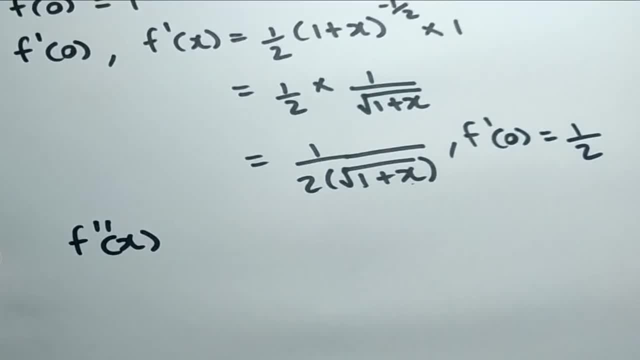 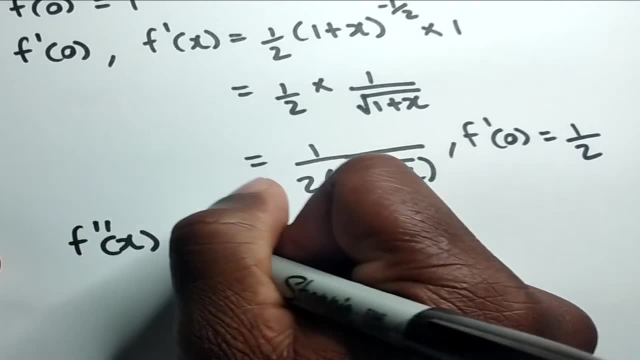 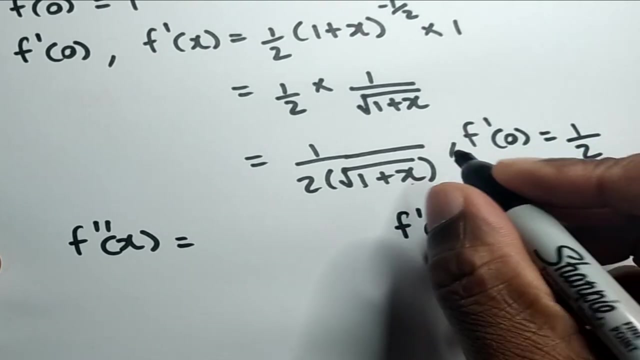 So what do we get if we differentiate this thing that we got? So we can rewrite this thing. So let's so want to obtain the function for this thing, But we can rewrite the function for the first differential of f, of x. And again, this thing is the same thing as what? 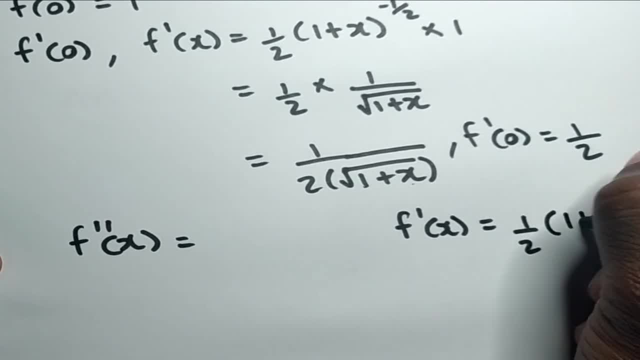 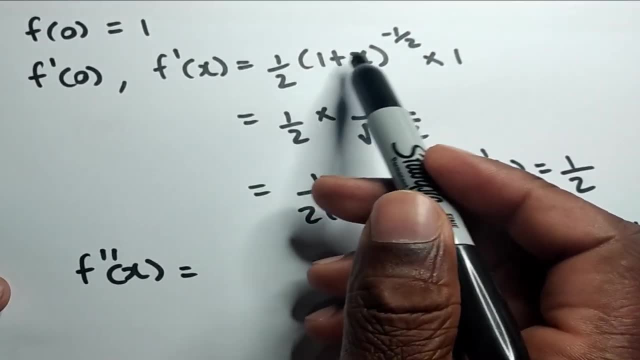 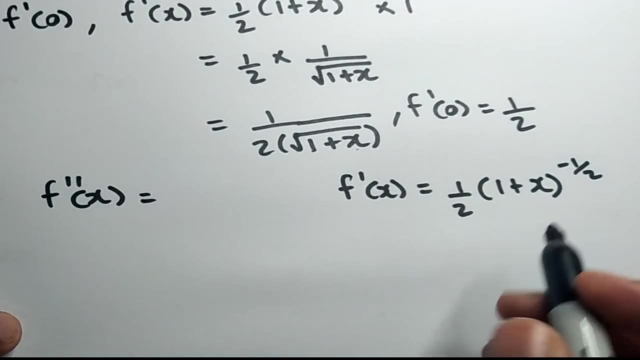 One over two in bracket, We have one plus x raised to the power of negative a half. All right, Same thing as we had right here. that we had right here. So this is the same thing as that. Now, if we should differentiate this thing, 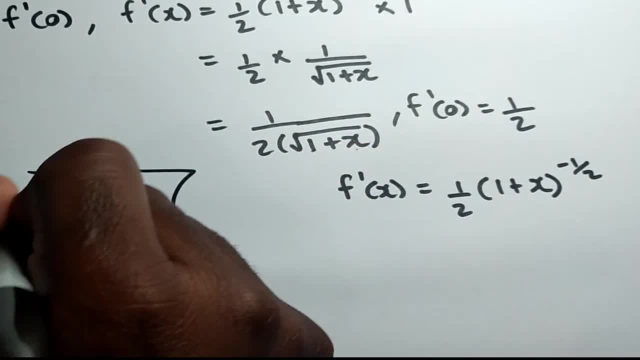 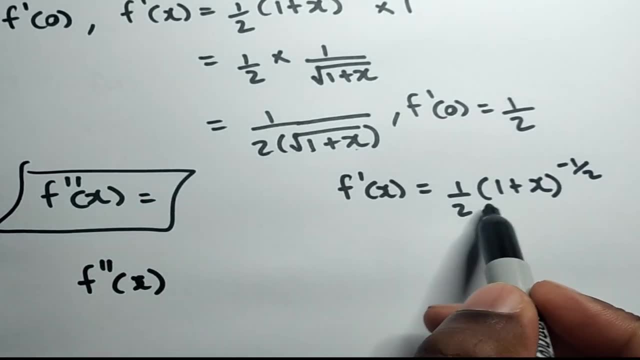 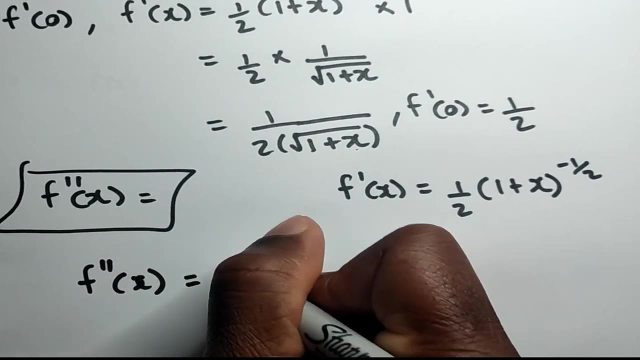 All right, And I'm going to come down a little bit. So if we should differentiate this thing, the second derivative- what we'll obtain is that we'll multiply this thing by the power, again So negative, a half times, this entire thing will will obtain what? 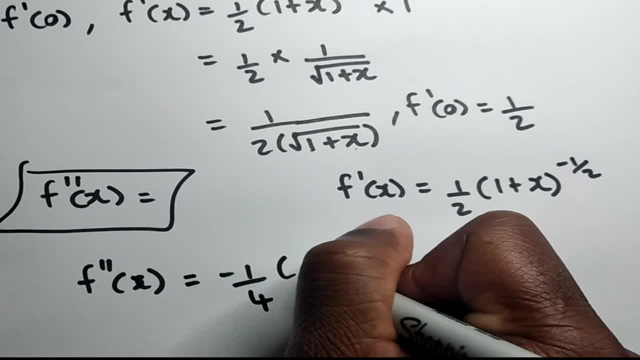 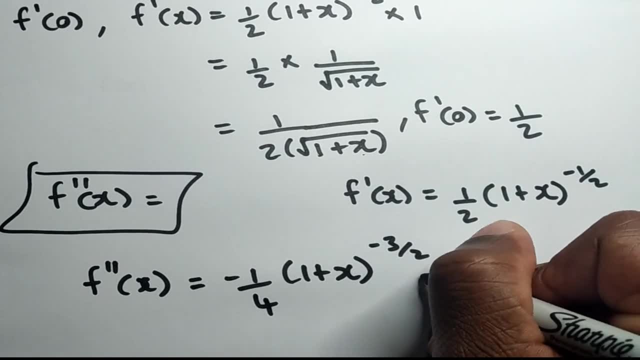 Negative one over four. in bracket We have one plus x minus one. from the power, We'll get negative three over two, And then we'll multiply this thing by the differential of the bracket, which is one. All right, So differentiate this thing using the chain rule. 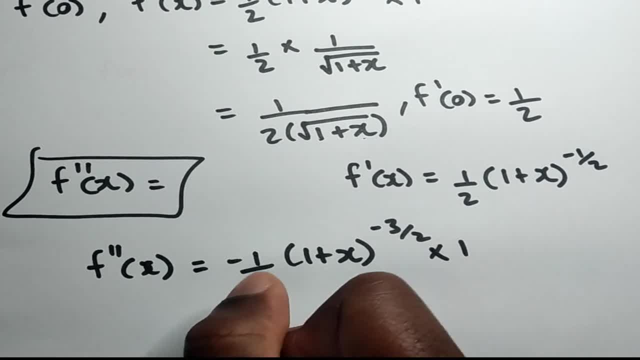 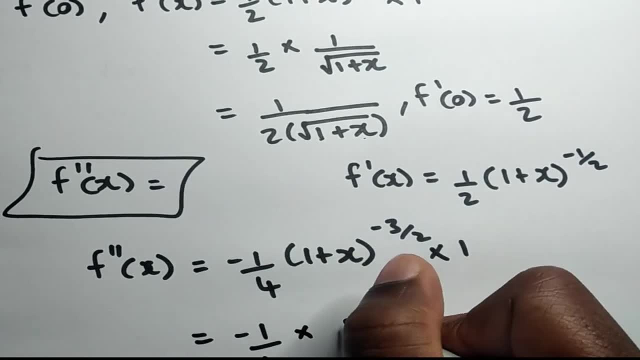 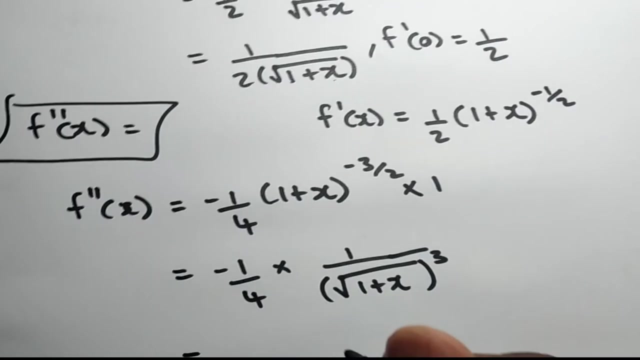 All right, So, and again, we can rewrite this thing. So negative one over four the same thing as negative one over four times one over the square root of one plus x, All raised to the power of three. All right, So we can do that and we can clean it up a little bit. so can clean this up some more. 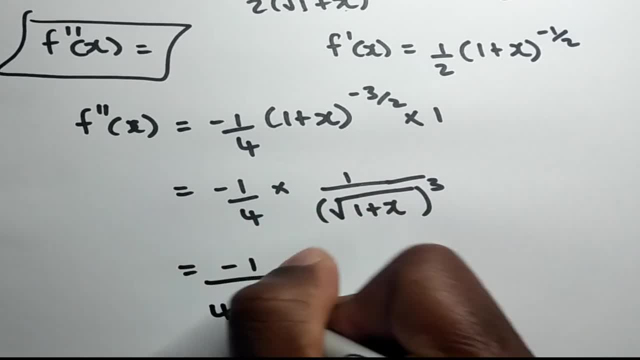 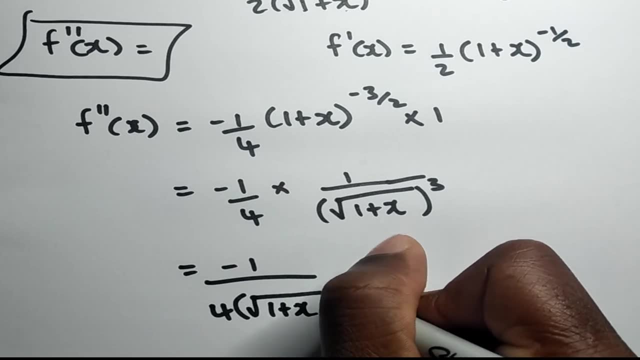 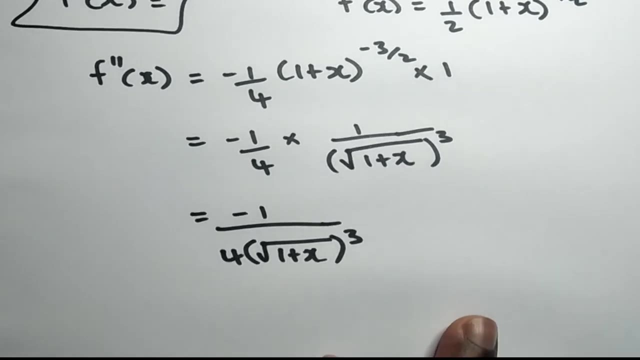 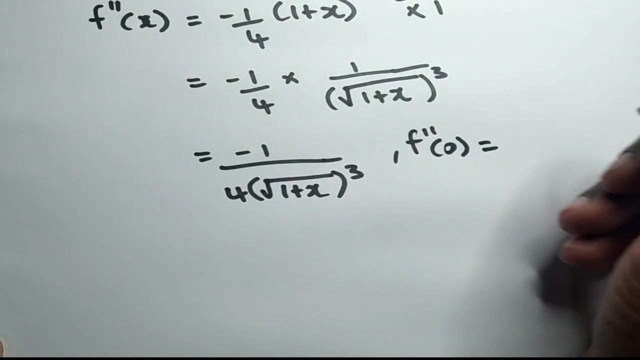 So this is same thing as negative one over four times one plus the square root of one plus x, raised to the power of three. All right, So where do we go from here? No, We want to find what we get if we substitute zero into this function. 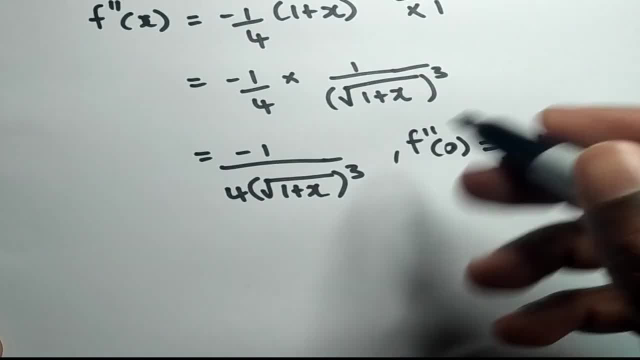 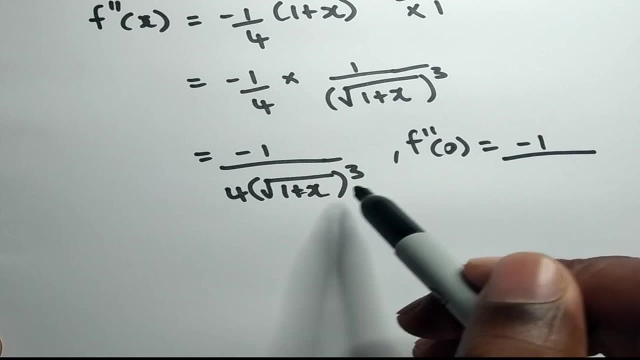 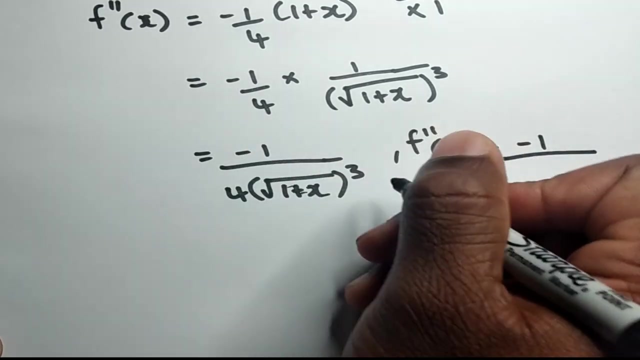 And that will give us negative one over. Let's see if I should substitute zero into this thing, What would we get? One plus zero, That's one. If one cube is one, four times one is one, So we'll end up with four times one, which is four. 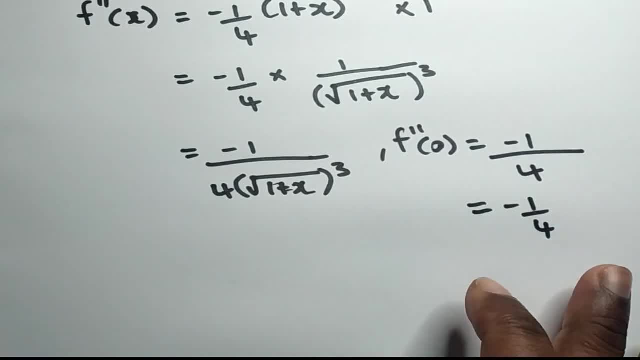 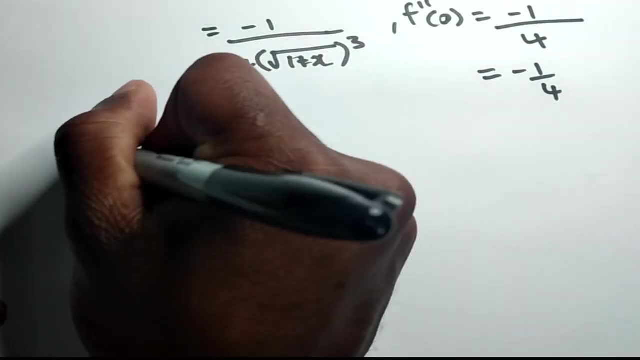 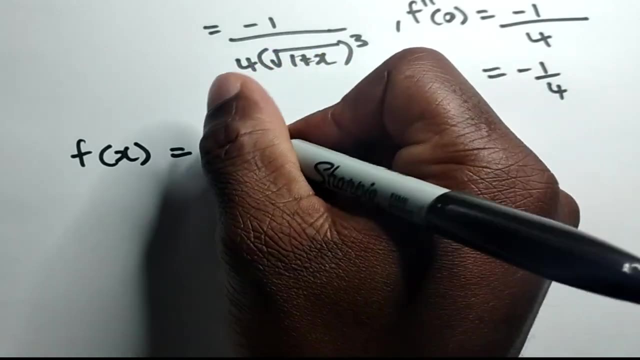 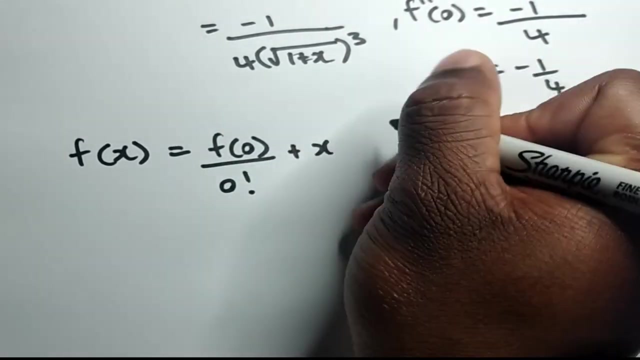 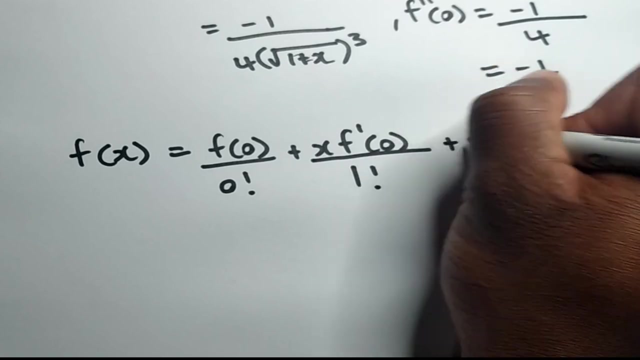 All right, So this is the same thing as negative four over four. All right, So that's what we'll obtain. So now we want to final step is to write this thing using the Maclaurin series expansion formula. So we'll have call the formula f of zero over zero factorial plus x times the result that we get when we sub zero into the first differential of f of x over one factorial plus x squared times. 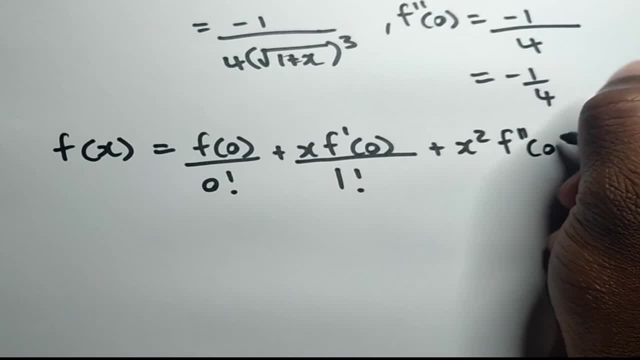 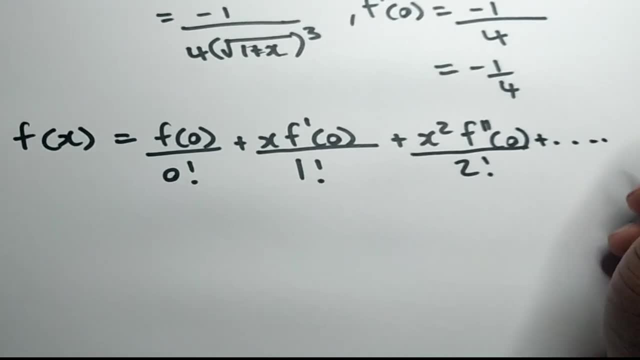 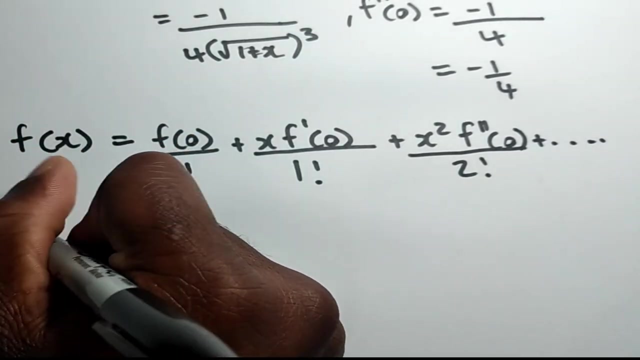 The result that we get when we sub zero into the second differential of f of x over two factorial. And, as always, we can always continue that thing, All right. So what we want to do now is to plug in the values that we got. 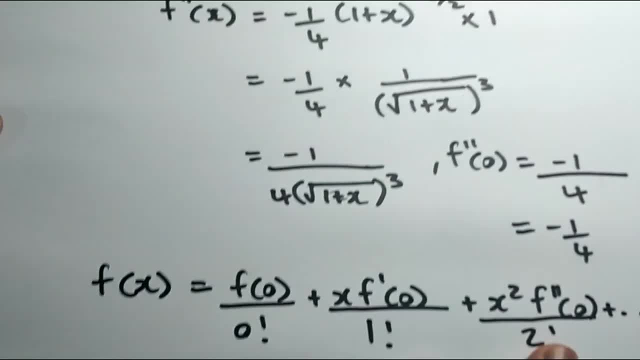 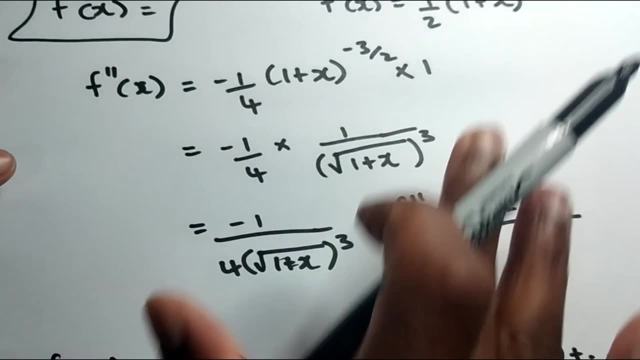 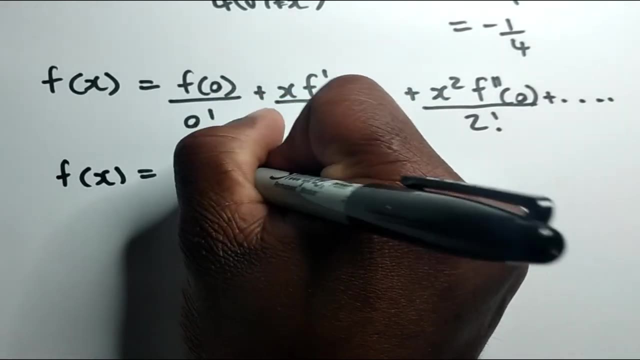 So f of x will be equal to what do we got for f of zero over? f of zero was one, So we got one right there. So we can have one over zero factorial, which is one, So that's one over one, So we can have one right here.